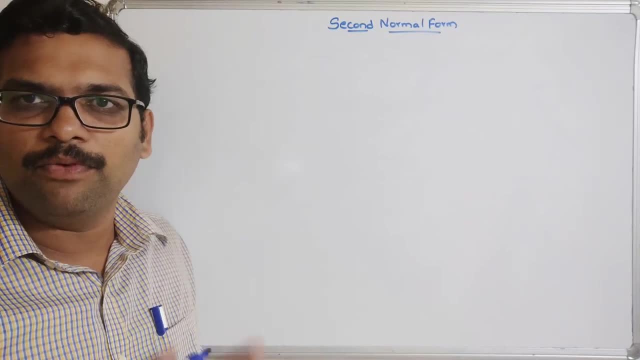 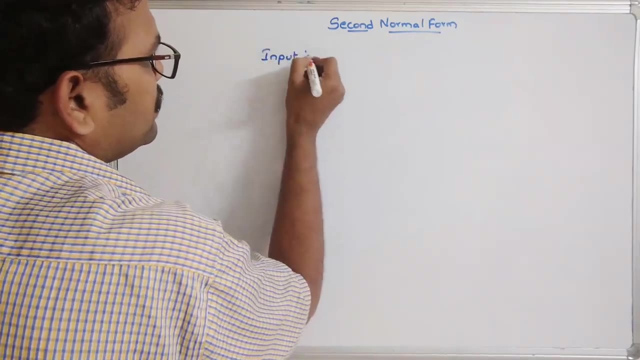 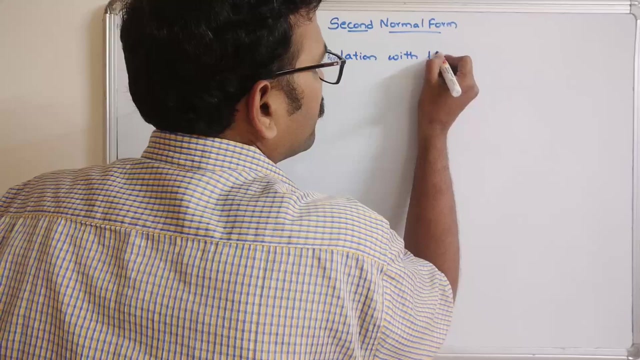 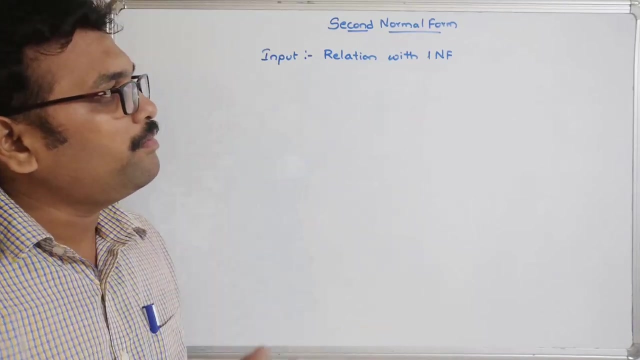 new rows and we have to avoid that. multiple values. And coming to the second normal form, the input for the second normal form is relation with 1NF. So that is the first constraint, that is the first condition. So if you want to check for the 2NF, so the relation should. 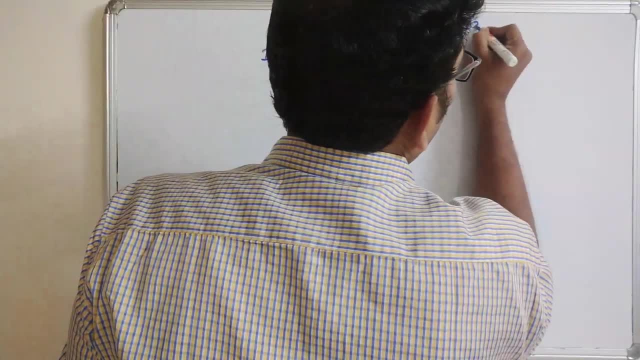 satisfy the 1NF condition, So this is also called as a 2NF. The second normal form is also known as a 2NF And the output, the output form, is 2NF, So the output form is 2NF. So 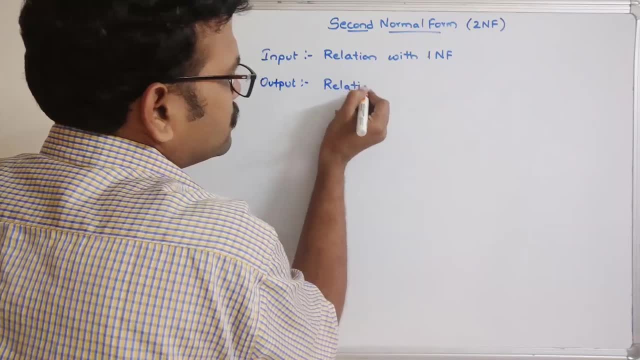 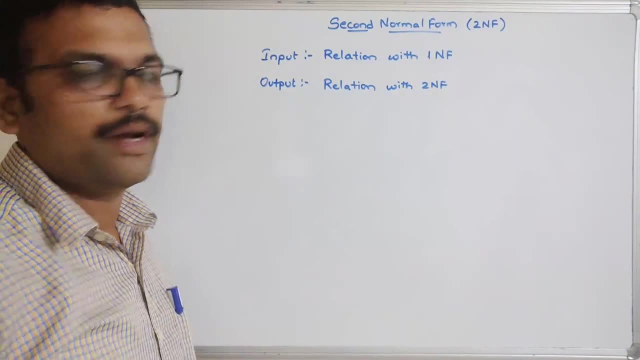 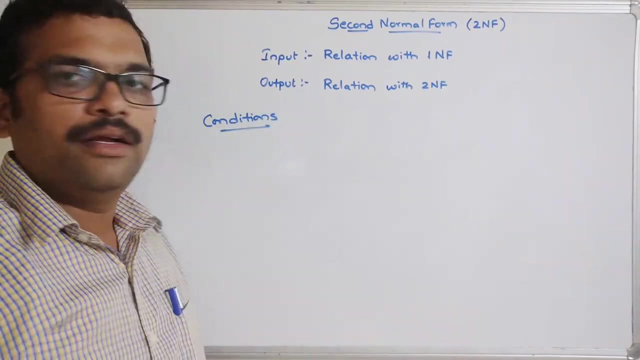 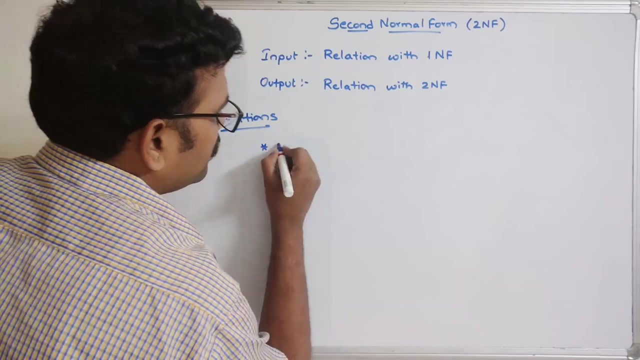 this one is relation with the 2NF. It is a relation that means the relation which satisfies the conditions of 2NF. Now we will see the conditions. Conditions need to be satisfied to say whether the relation is in 2NF or not. So the first condition is the. 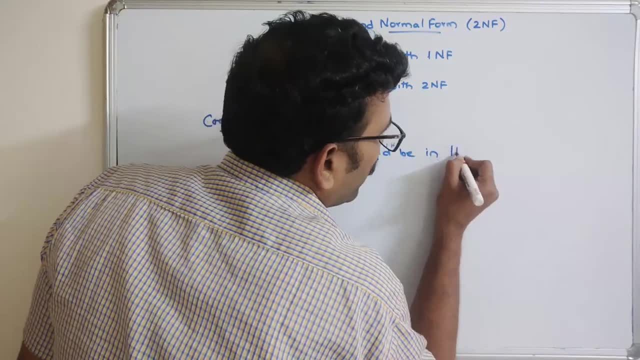 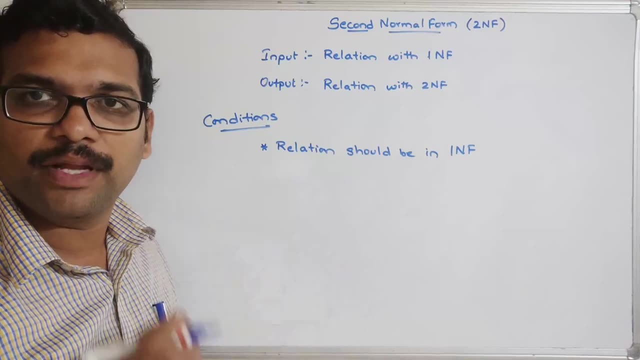 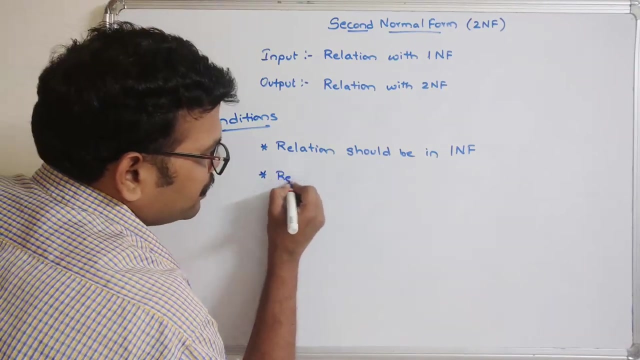 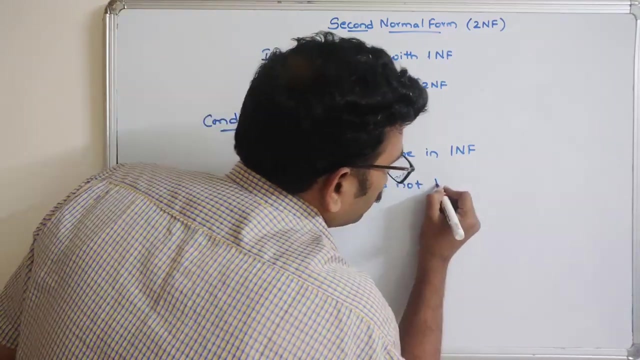 relation should be in 1NF. So first we have to check whether the relation is in 1NF or not. So if not, first we have to achieve the 1NF. That means we have to make the relation in 1NF. That is the first condition. The second condition: the relation should not have partial 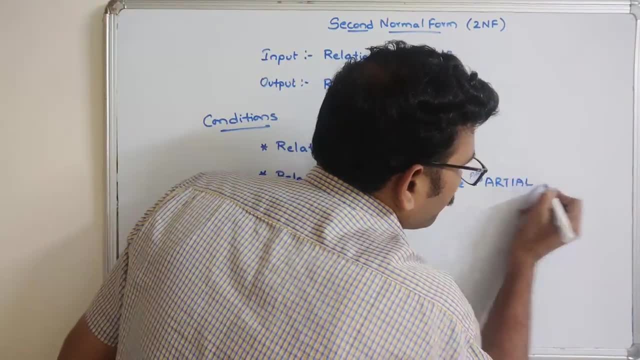 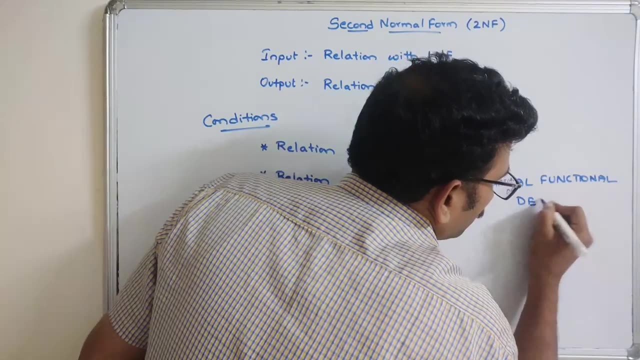 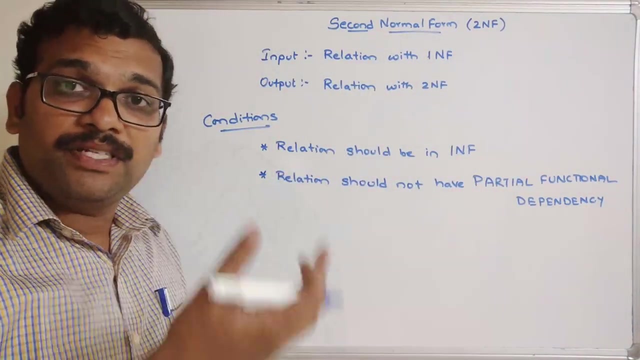 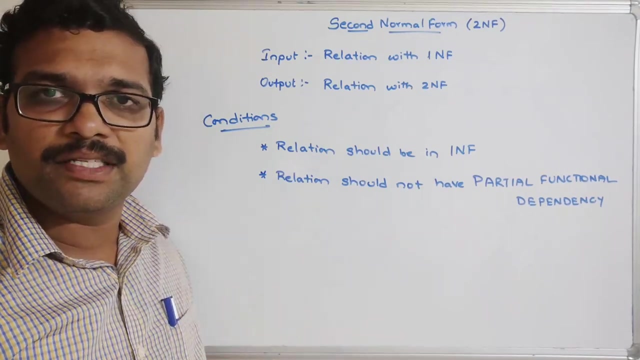 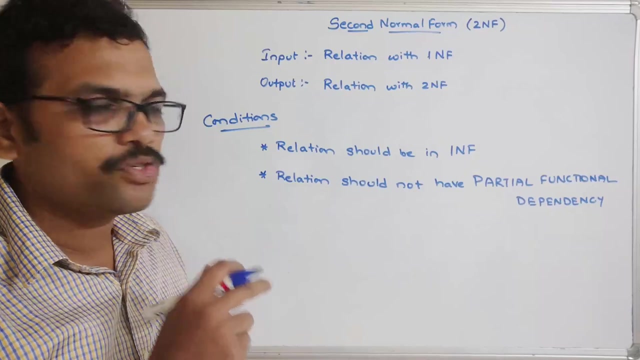 functional dependency, Partial functional dependency. So in the previous sessions we have discussed about the functional dependencies And in that video we have discussed about the two different types of functional dependencies, That is, a fully functional dependency and a partial functional dependency. So I will post the link in the description So that first go. 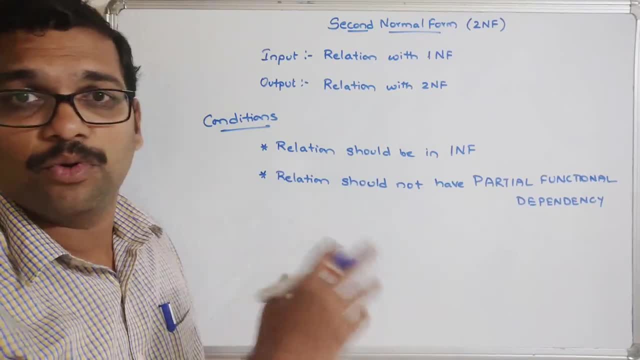 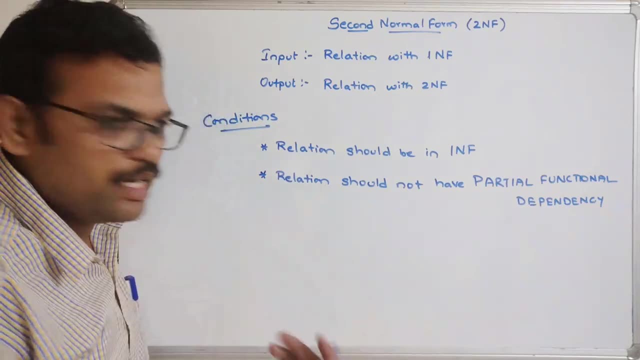 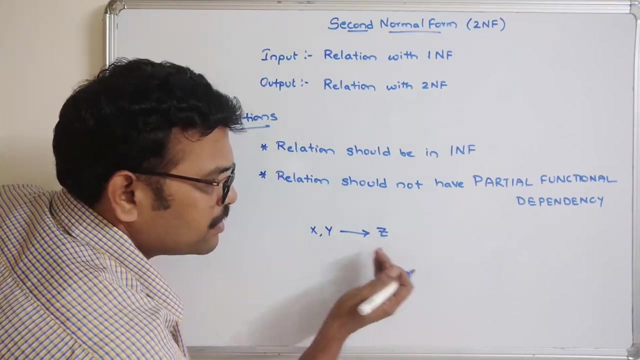 through that one And then you will get a clarity about the partial functional dependency. So at a glance I will just recall the concept. So, for example, if any functional dependency in this format, some x, comma, y tends to z, So this we call it as a determinants and this is a dependent. 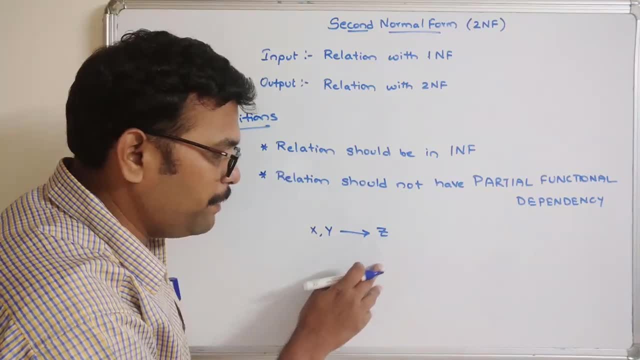 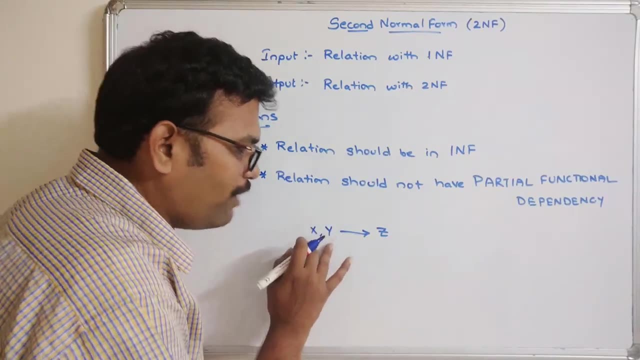 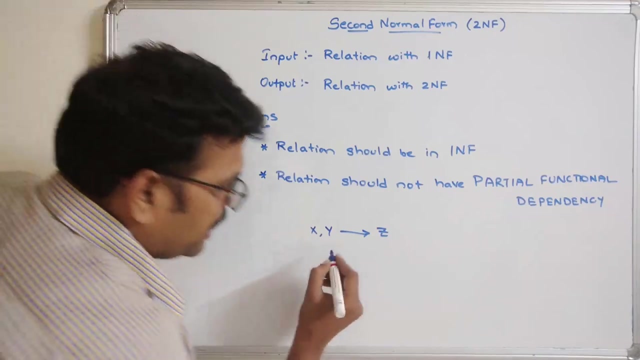 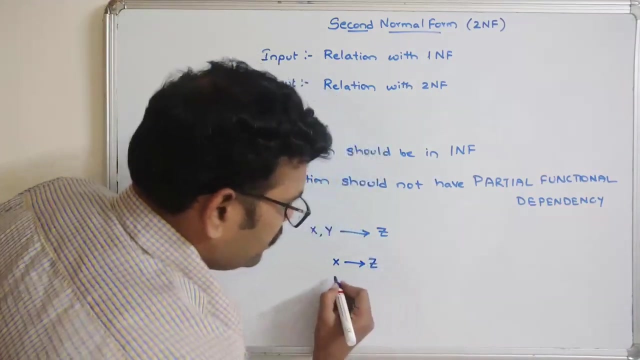 So that means we can say z is functionally dependent on x comma y. So that implies by knowing x and y values, With the help of x and y values, we can determine the z value from the relation. So if x comma y tends to z is a functional dependency, then if it satisfies any one of these conditions, 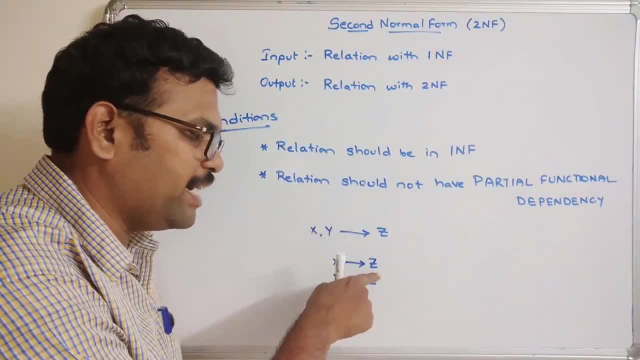 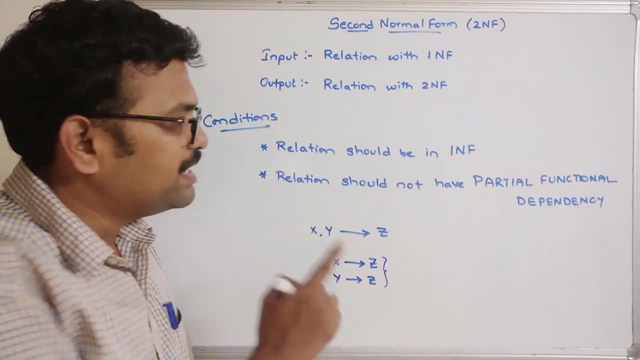 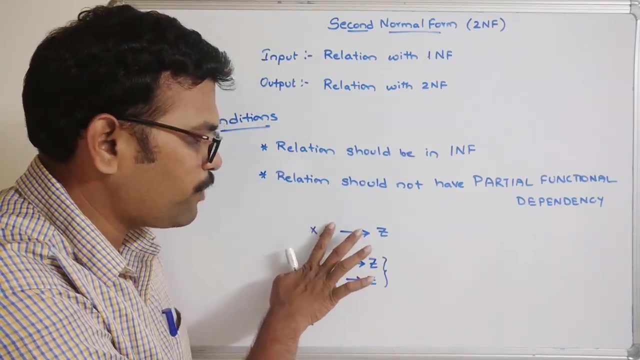 that means if you know the value of x, if you can determine z. or if you know the value of y, if you determine z. So any one functional dependency is true. That is a partial functional dependency. Okay, so here we are removing one attribute from the determinant, And still there is a functional. 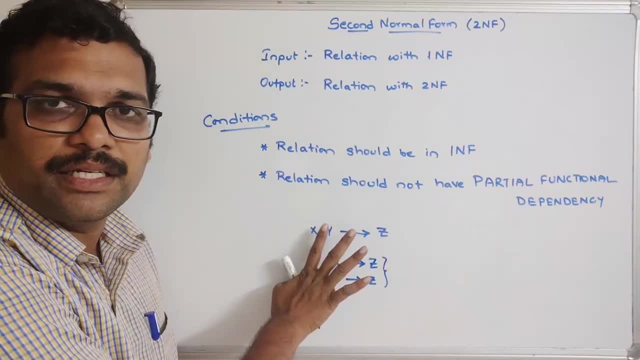 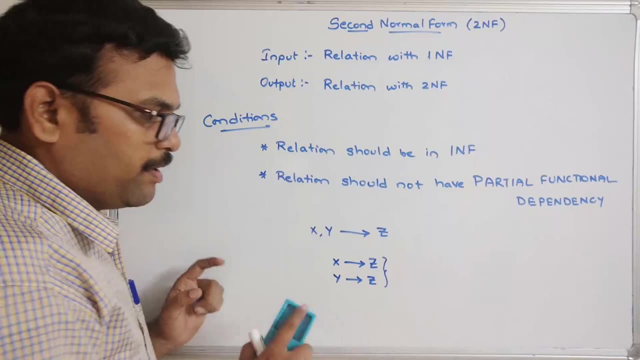 dependency exists that we call it as a partial functional dependency. right, So that we have discussed in the previous sessions. I will post the description, So just go through that one. So this is the thing. So if any one of this functional dependency, if any one of these one is in functional 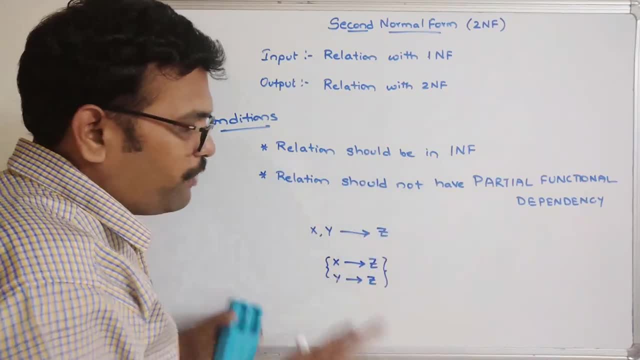 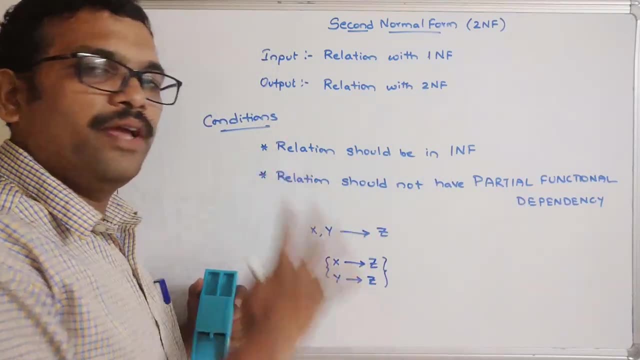 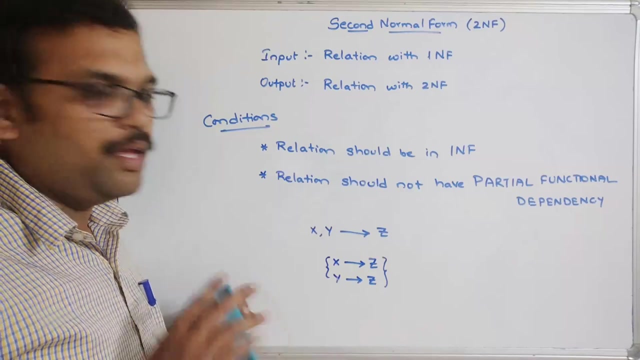 dependency. we can say it is a partial functional dependency. So we have to find out this one, And we have to find out whether there is a partial functional dependency or not. If so, we have to remove that partial dependency by decomposing the relation into sub relations. Okay, so the two conditions to satisfy. 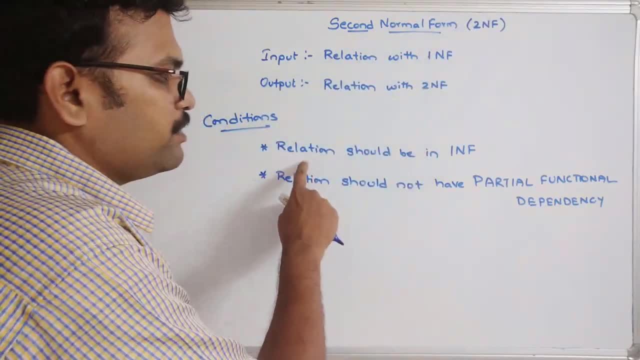 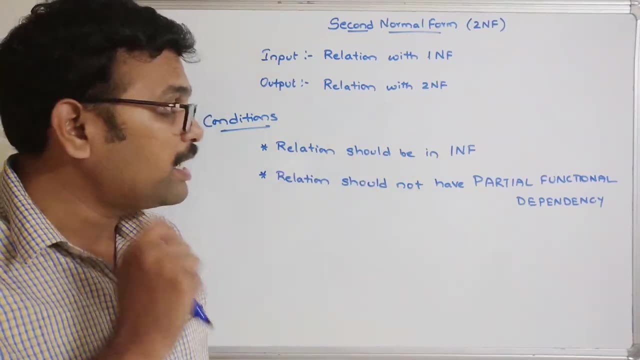 whether the relation is in 2NF. So that is the first of the relation should be in 1NF And then the relation should not have the partial functional dependencies. Now let us check with a small example. See, let us take this example. 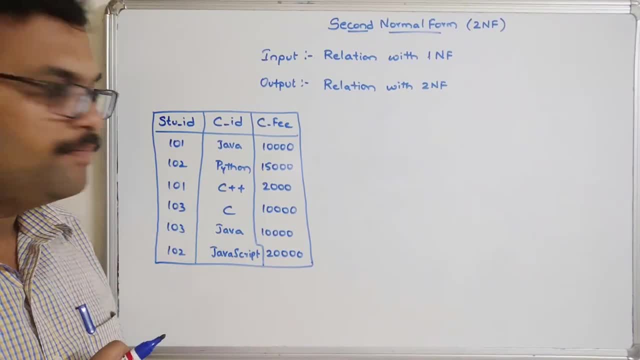 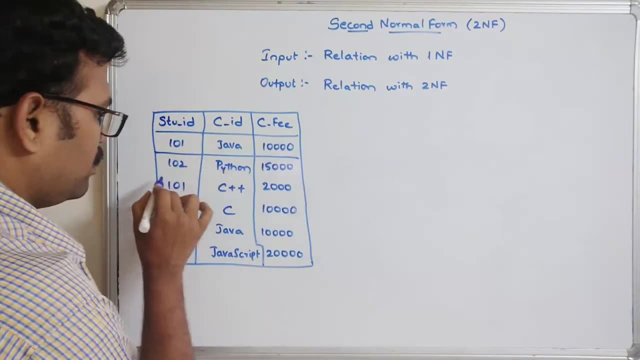 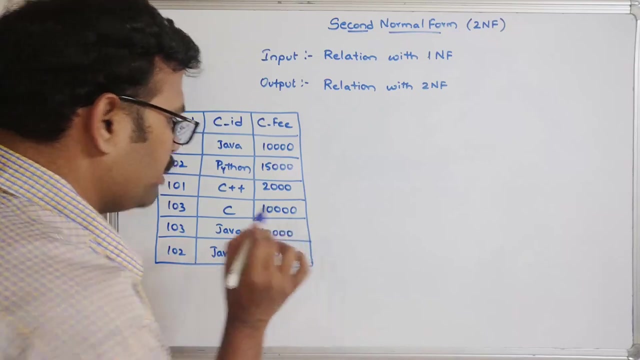 So there are three attributes in this particular relation. So there is a student ID course, ID course fee, Right? So first we have to check whether there are multi-valued attributes. that means multiple values for any single attribute, right? So you can observe, for every column we are having only one. 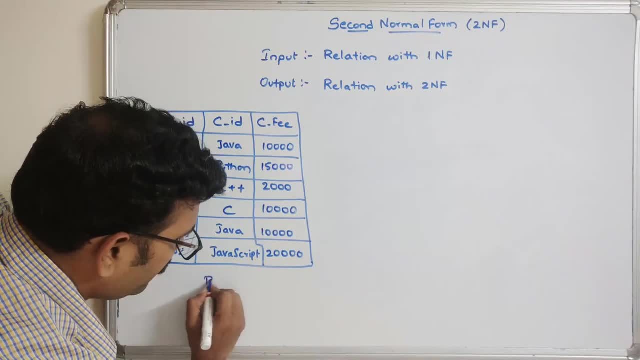 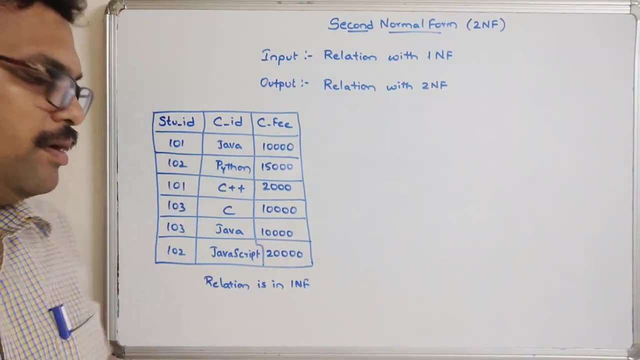 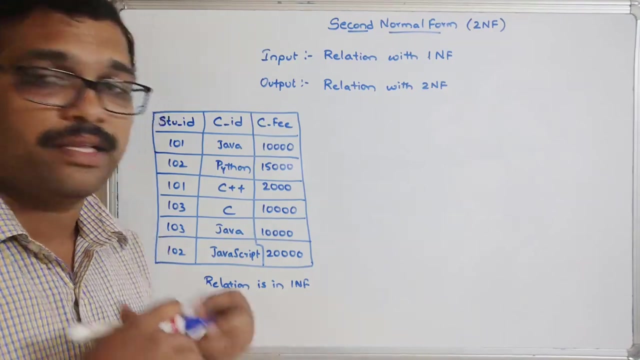 attribute. So that implies this is in this particular relation, is in 1NF, 1NF Right. So we have to check whether this relation is in 2NF or not. So for that we have to find out the functional dependencies and we have to find out whether there are any partial functional. 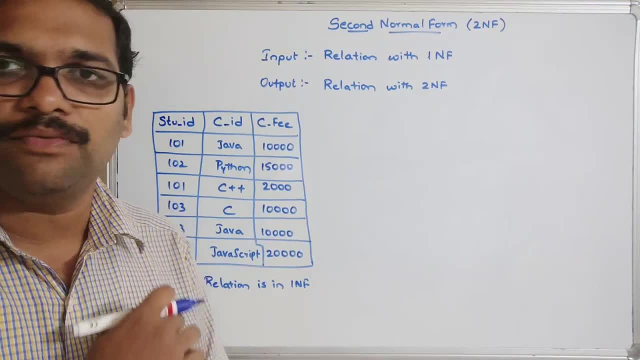 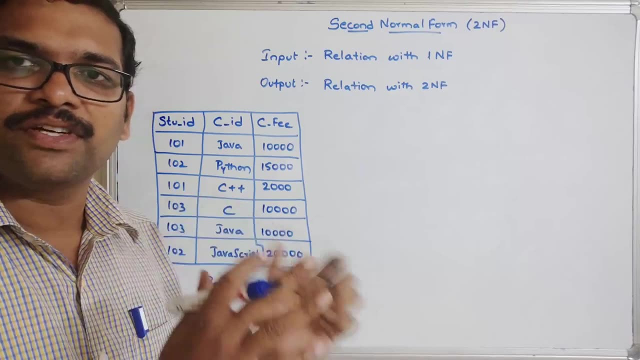 dependencies. So if there are any partial functional dependency, automatically we say that the relation is not in 2NF, So that we have to avoid that partial functional dependency. That means we have to remove the partial functional dependency so that this relation will become the 2NF That 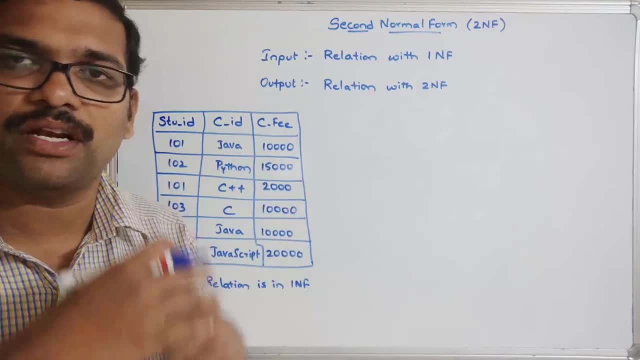 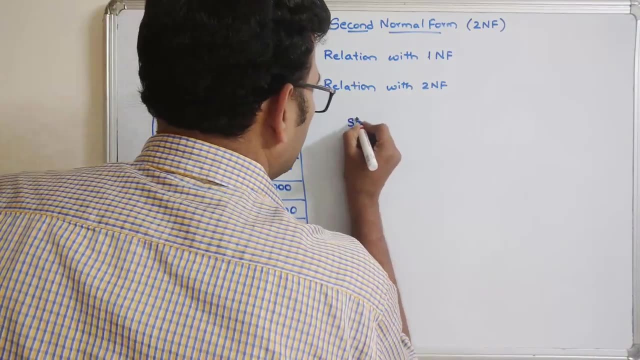 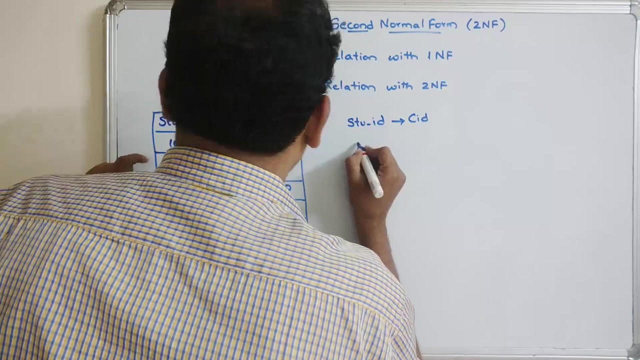 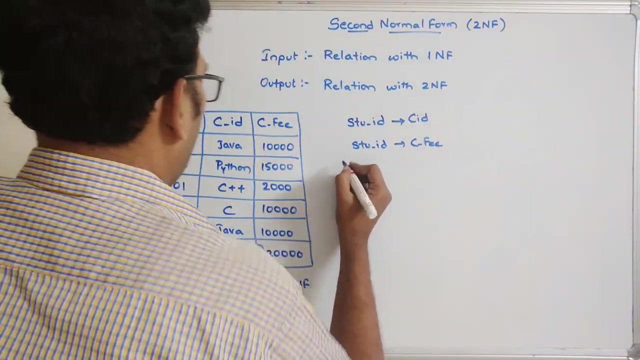 means we have to decompose this relation to the sub relation so that it will be in 2NF. Right Now let us check with the functional dependencies. So I will take the functional dependencies. So student ID tends to course ID and student ID tends to course fee And course ID tends to course fee. 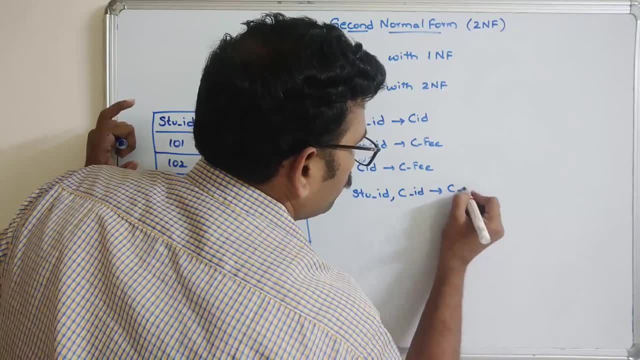 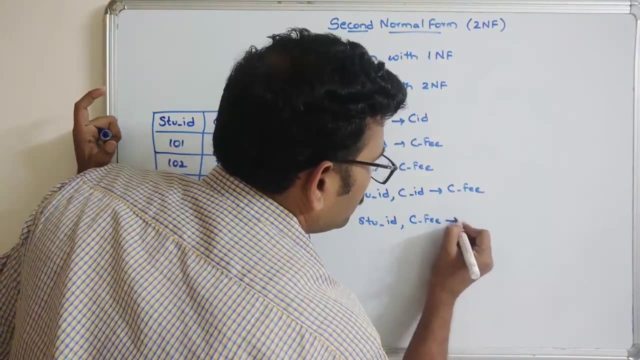 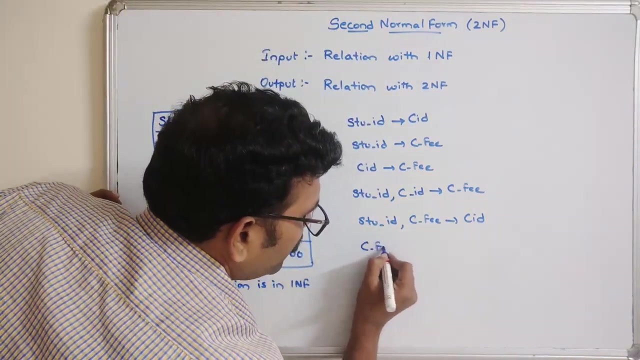 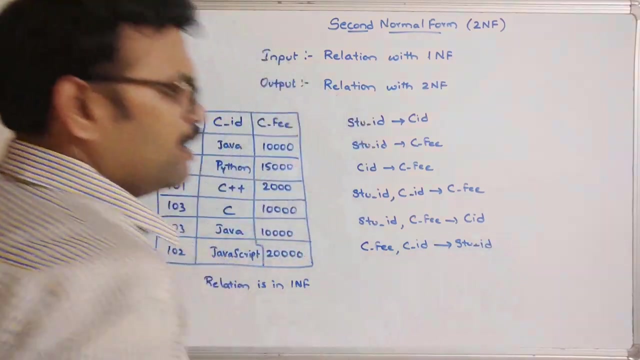 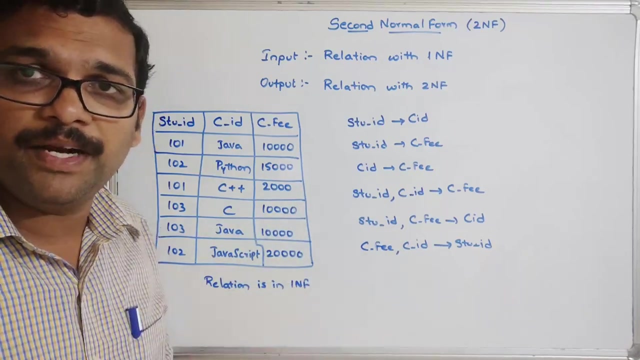 ID tends to course fee, student ID. course fee tends to course ID, course ID right and then course fee comma. course ID tends to student ID. so these are the possible cases. now we can check whether there is a functional dependency or not for all the things. so functional dependency means on the left hand side. 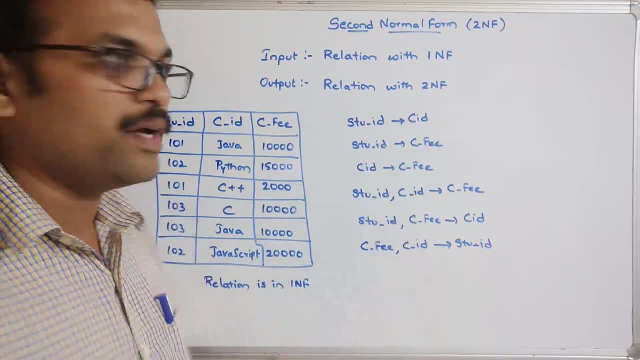 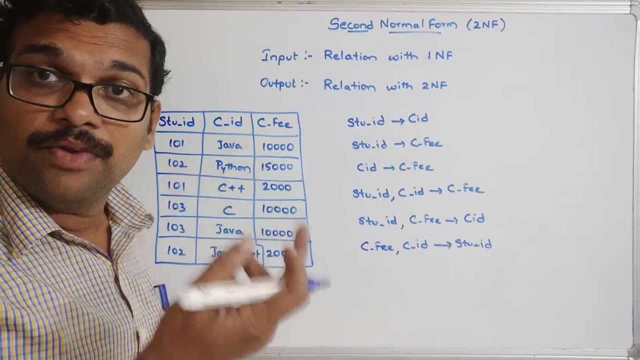 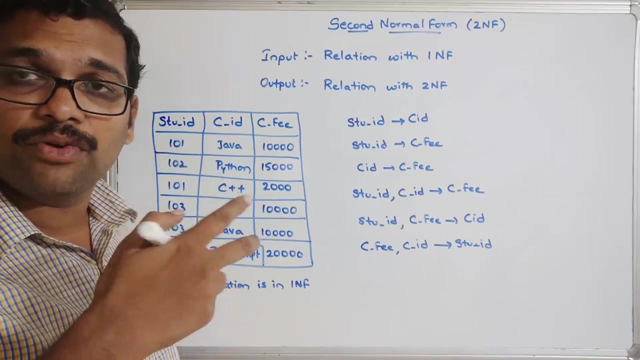 the determinant and right hand side is the dependent. whether CID is dependence on the functional, dependent on the determinant or not, that means we have- we have studied about this functional dependency in the previous session. so we have to check for one constraint: that we have to consider two random tuples. so 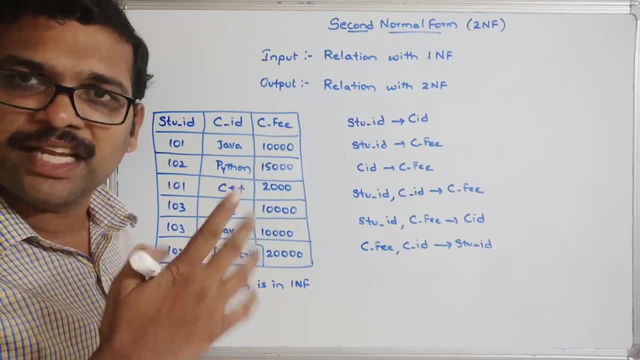 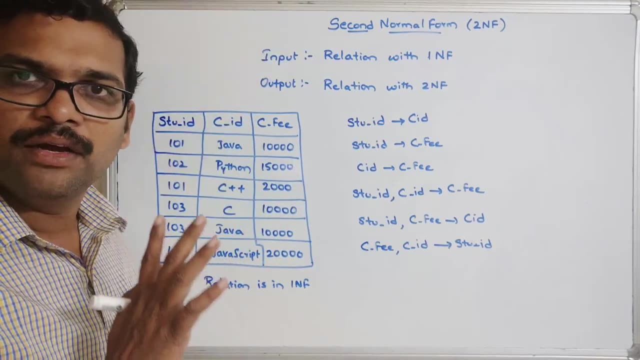 that the X value are equal. if both the tuples are having the same X value, the corresponding Y values are also equal to the same value. so we have to check for which these two values are equal to the same value. also to be same, then only we can say there is a functional dependency. so once just go through the functional 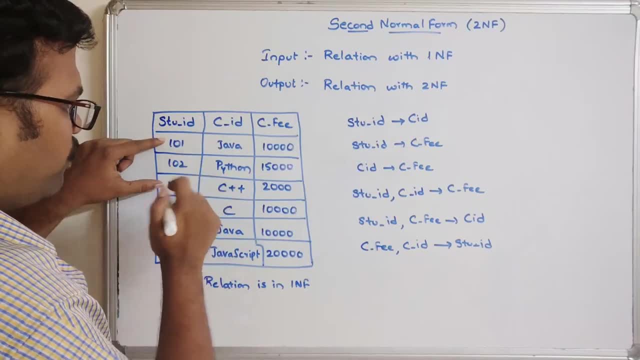 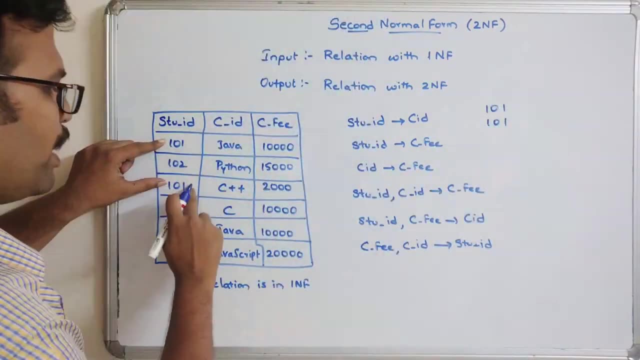 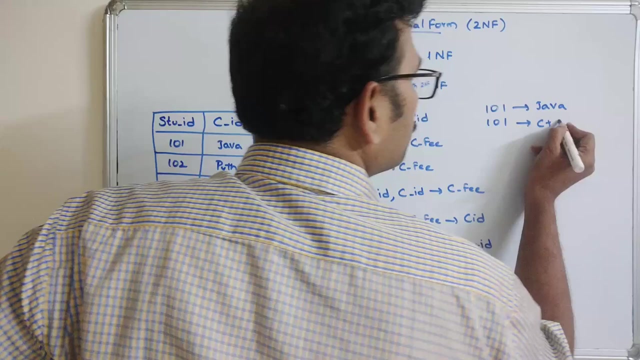 dependency concept video, right. so here let us take student ID and course ID. student ID: let us take a two to pose 101 and 101. so here 101, let us take 101 and 101. two toples X value is 101, 101 and here we are getting Java as a course ID. and 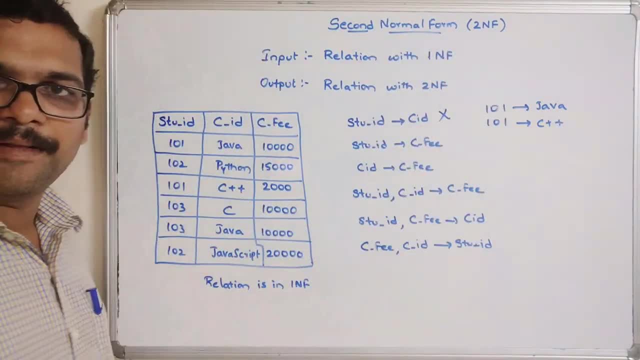 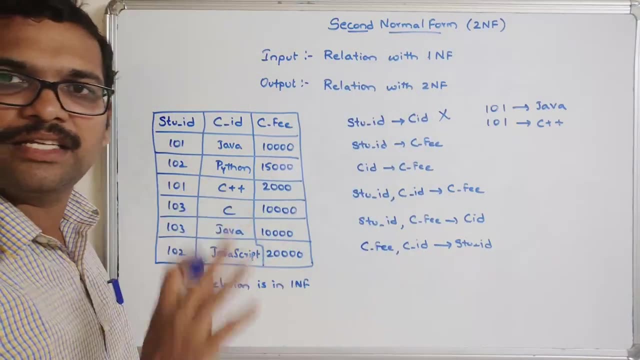 here we are getting C++ as a course ID, so there is a tendency, so we can test for that one. all right now, let us see how will it work. can't say this is as a functional dependent, right? so considering two different x values, there should be corresponding y values. then only we can say that it's a functional dependence. 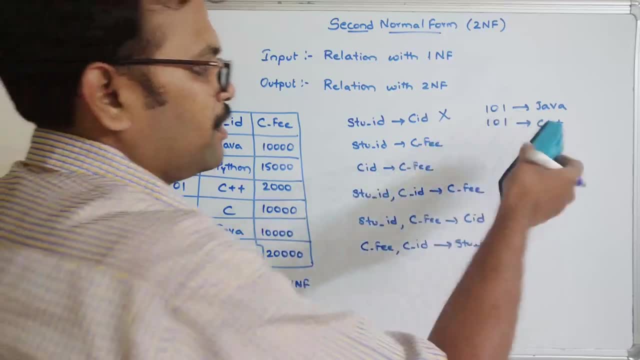 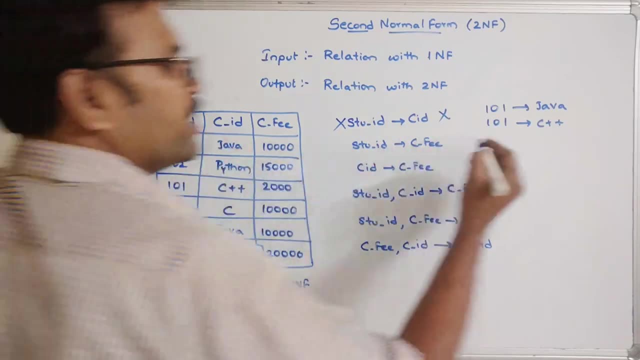 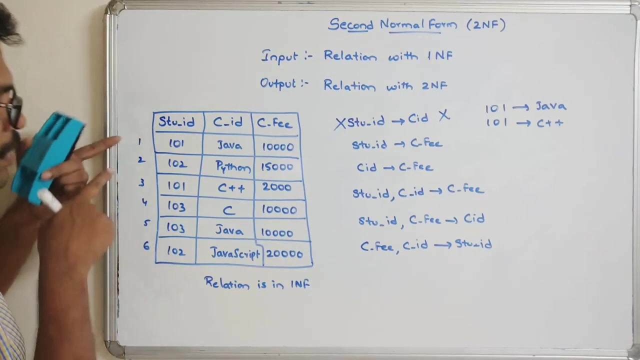 so here there is no functional dependency. so this is not a functionally dependent. now let us take this one student id and course fee student id again you can check. so the first tuple and second tuple. so here i will write it in numbering, okay, so you'll be understanding. so consider the first. 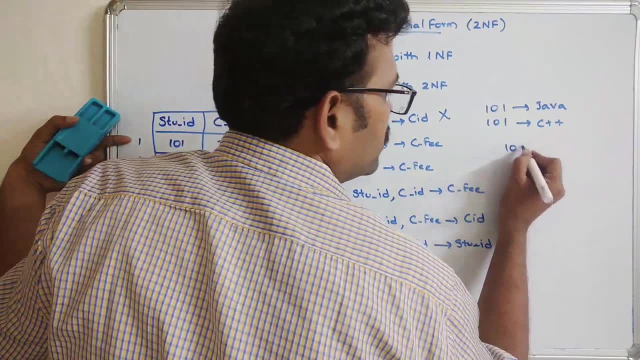 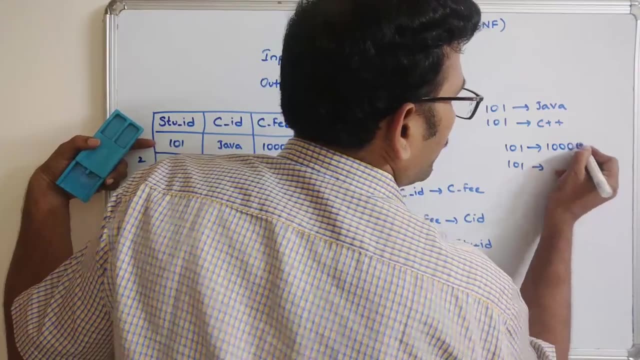 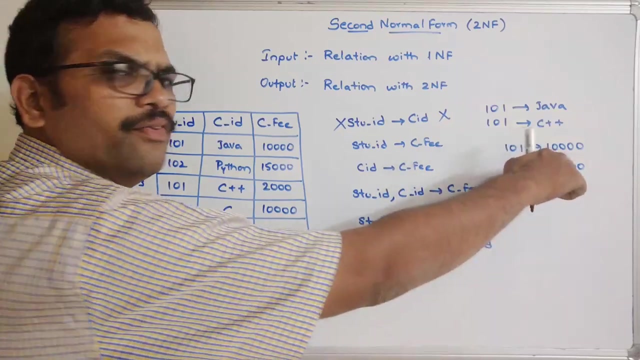 tuple and the third tuple. so again we are having 101 and 101, so corresponding course fee. 101 course fee is some 10, 000 and 101 2000. so here for the same x value we are getting different y values. so this is also not functionally dependent. so we can't say this is a functionally dependent. 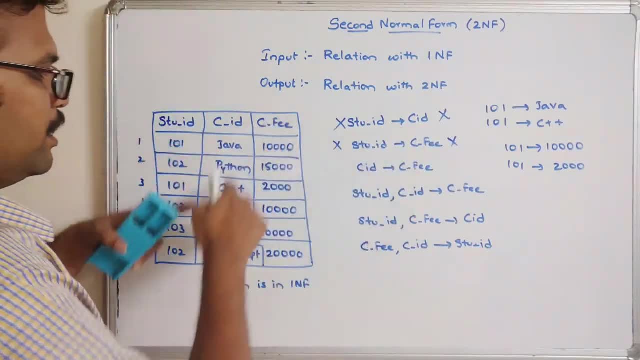 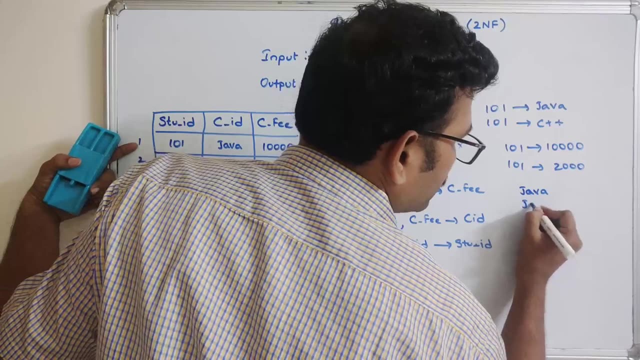 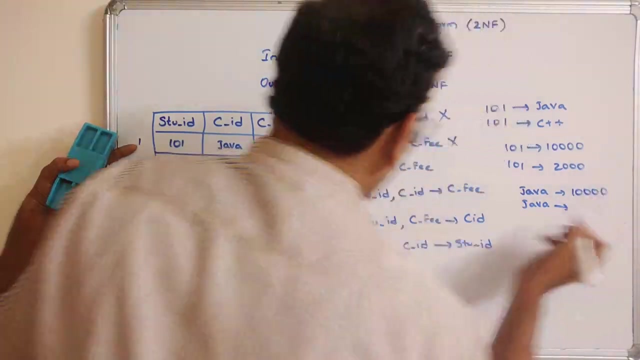 right, consider one course id and course fee. so consider: see first one and fifth one. so first one and fifth one. we are having the x value as java. so what is the corresponding y value here? 10 000 for the first triple and coming to the fifth triple, again it is a 10 000. yes, so both are x values, both x values. 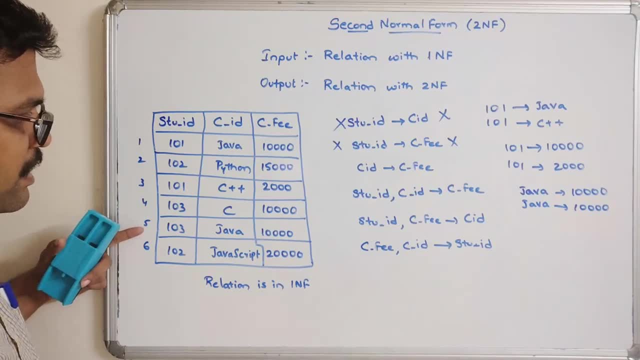 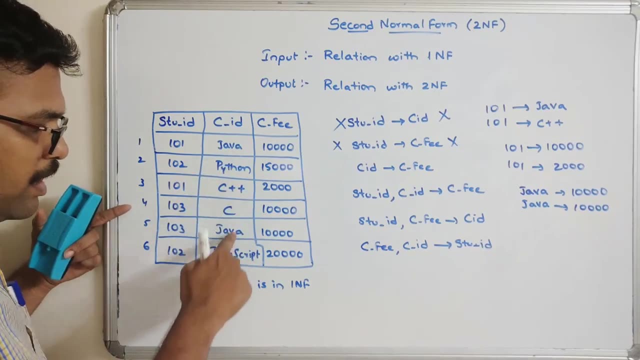 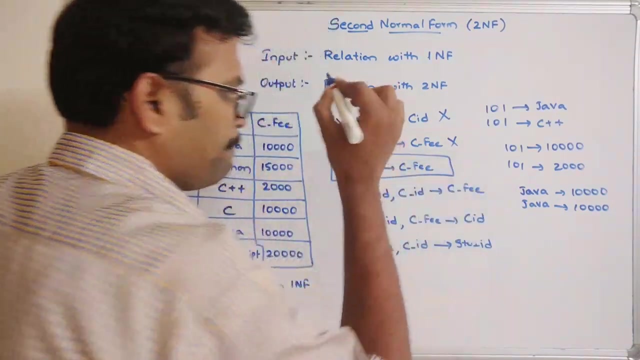 are same and corresponding y values also same. consider: yes, so that's the only thing we have that is repeated in the table: java and java. so all the remaining are unique, so we can say this as a functionally dependent. okay, so this is one functional dependent, right? and now let us consider. 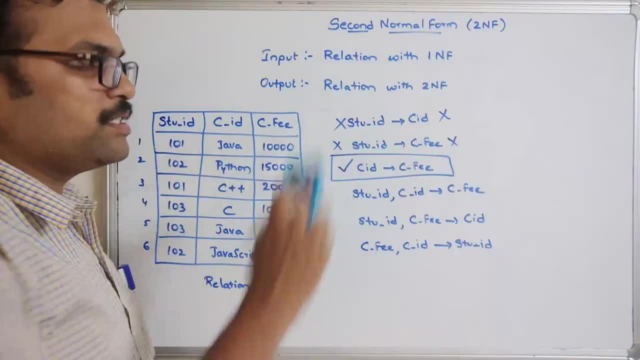 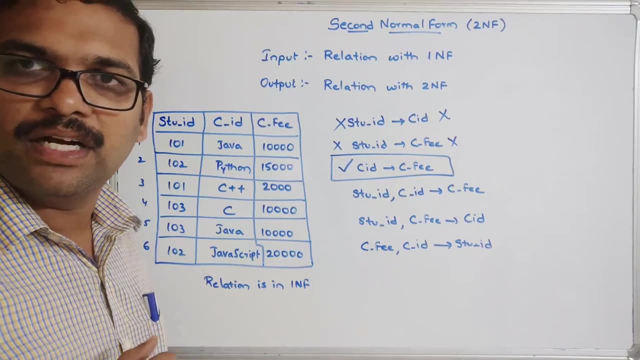 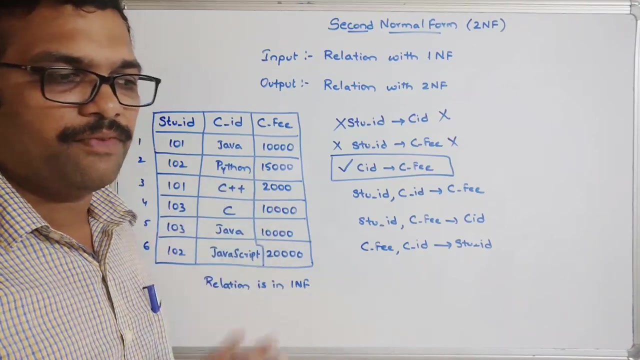 these things. so we let us bother about these functionally dependents because we have to eliminate the partial functional dependency. so when we will get the partial functional dependency? if the determinant is having some set of attributes, then only we can say we can. we can say the partial functional dependency and the full functional dependency, but here the determinant 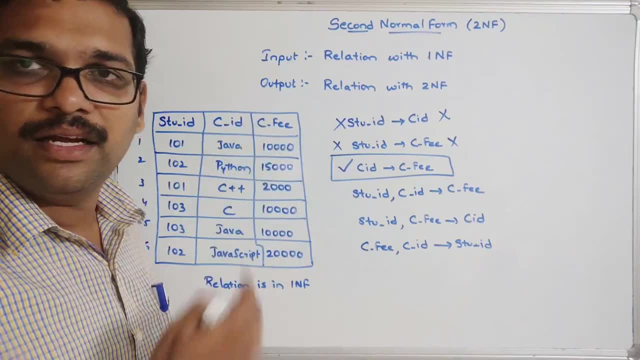 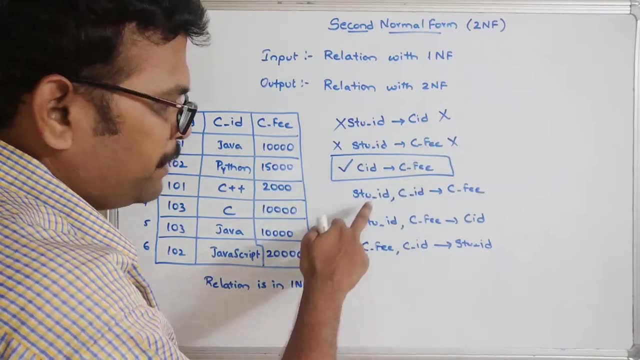 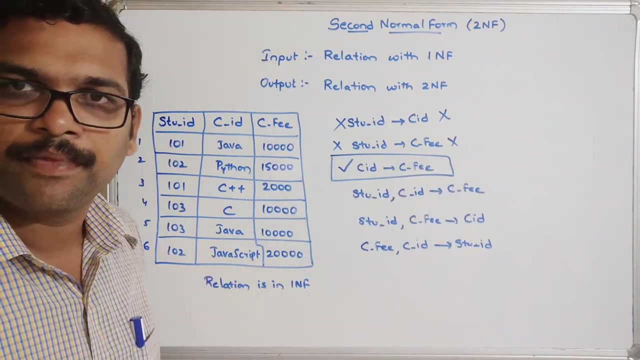 is only one attribute, so we can't say it is it has a partial or full functional dependency. okay, there will be no partial dependency, it's a full functional dependency. now, coming to this, one student id and course id combinedly determines the course fee. okay, so don't think it has a two. 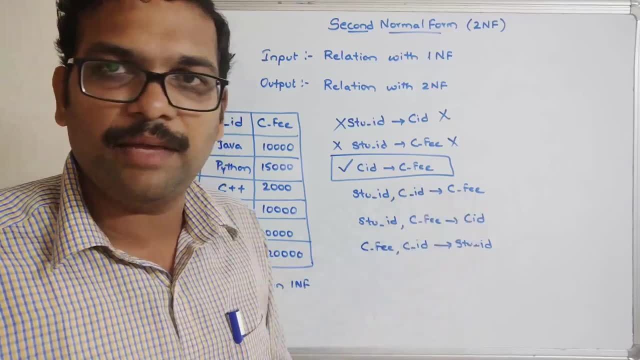 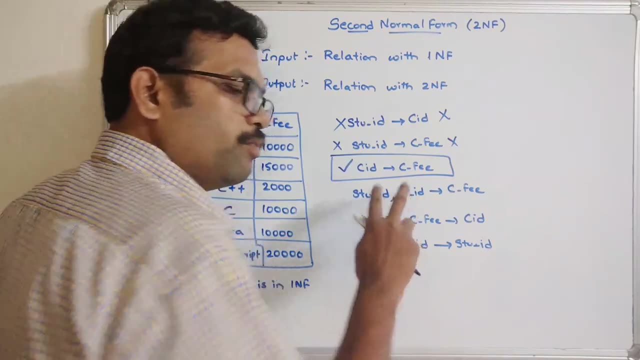 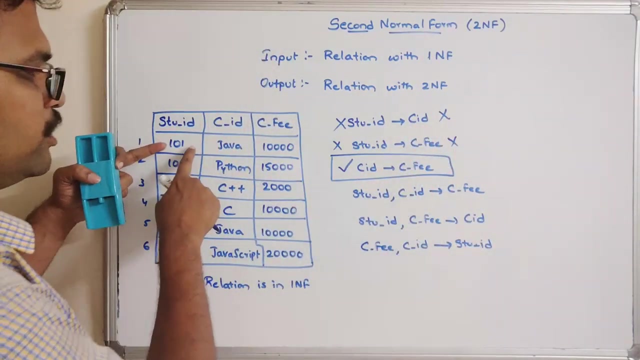 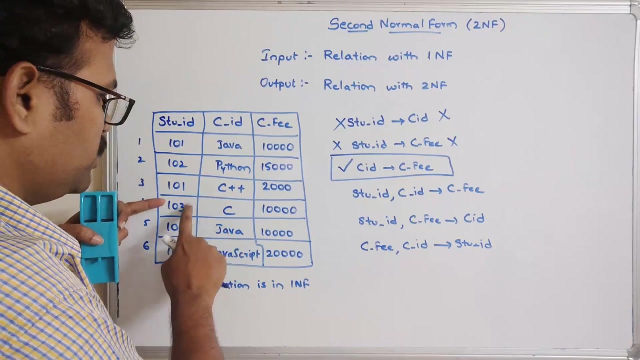 different attributes, okay, two different attributes giving to the same thing. so this, the meaning of this particular functional dependency means, by knowing the student id and course id, the combination of student id to course id. it should give the value of code speed. let us check. so: 101 student id, java, okay. 102 python, 101 c plus plus 103 c, 103 java, 102 java state. so all. 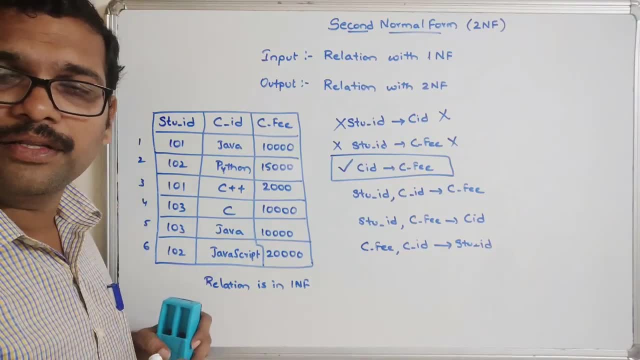 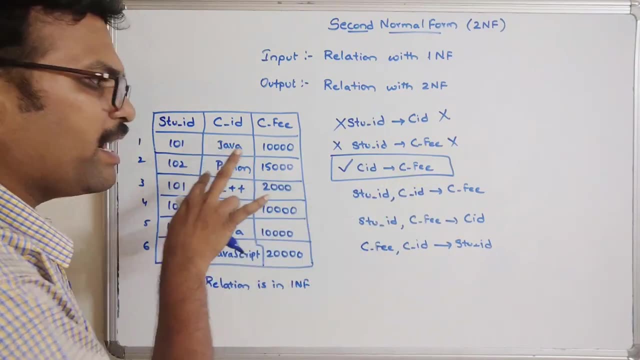 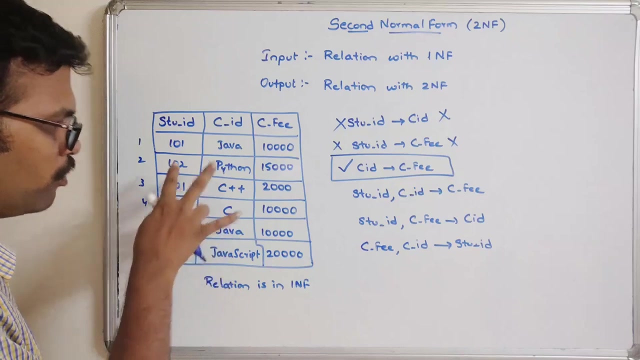 are different, all are different, all are unique. there is no repetition. so we have to consider these two, student id and course id. so is there any relation? i mean, is there any redundancy for these two? 101 java- is there any 101 java? there is no thing. 102 python no. 101 c plus plus no. 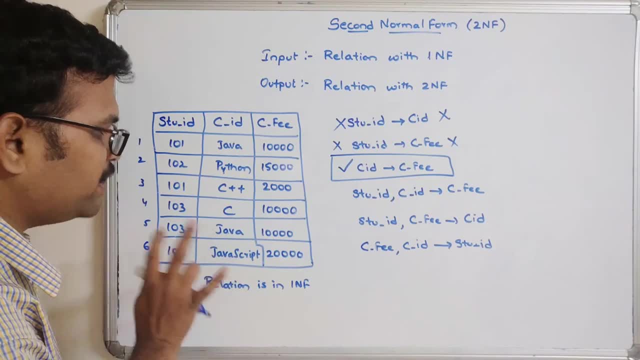 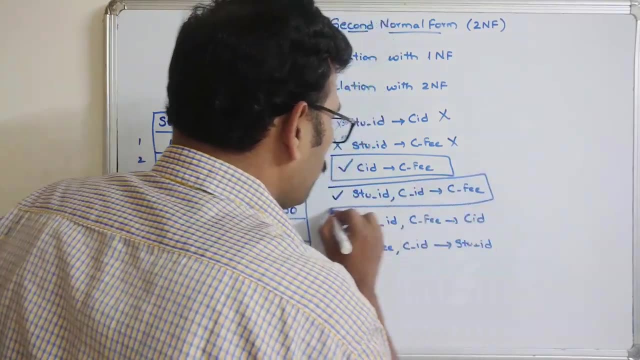 one zero c, no one zero three. and java: one zero two and five. uh, javascript, there's no redundancy. so we simply we can say this is also a functionally dependent. this is also also a functionally dependent because by knowing these two things we can get the code. 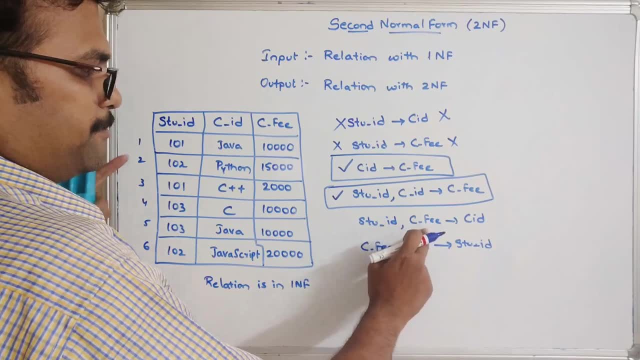 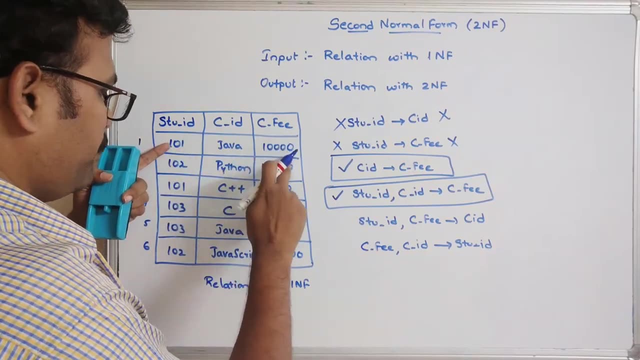 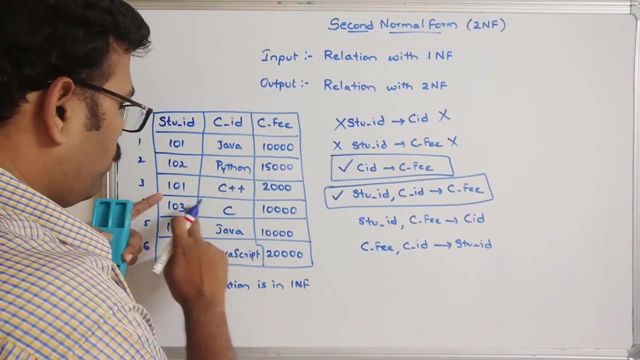 speed uniquely. and coming to the student id and course fee: student id and course fee: check student id and course fee. 101 and ten thousand. is there any repetition for 101 and ten thousand? no, no one. zero two and fifteen thousand: no one zero three and one one zero three and ten thousand. 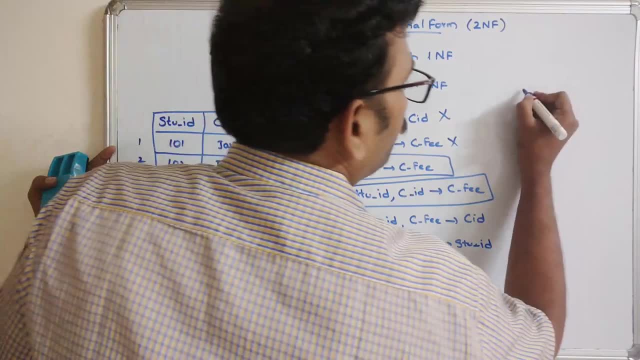 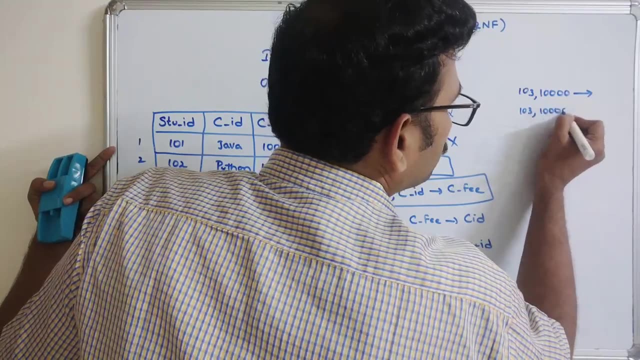 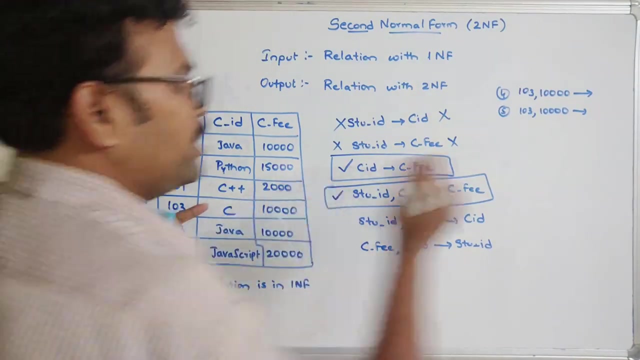 yes, see one zero three and ten thousand four and five. so four and five, one zero three with a ten thousand, one zero three and with ten thousand. so you can observe the fourth tuple and fifth tuples, fourth, 2 and 5 tuple: 1, 0, 3, 10 000. 1, 0, 3, 10 000. so here we are having some c and here we are. 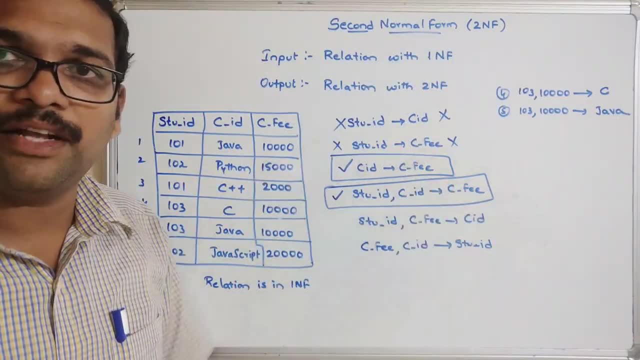 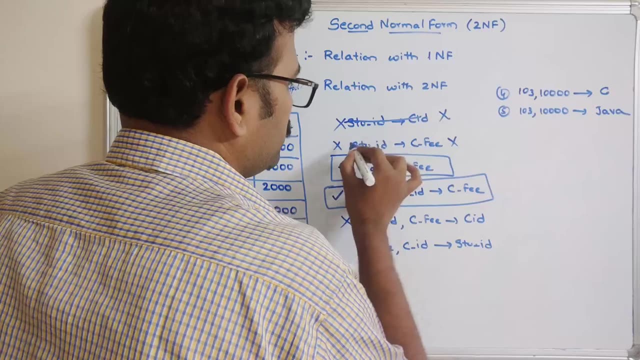 having some java, so same x value gives a different y values. so we can't consider it as a functional independence. so this is not a functional dependence just because strike off. so this is not. this is not and this is also not a functionally dependent. coming to this, one voice: 1. 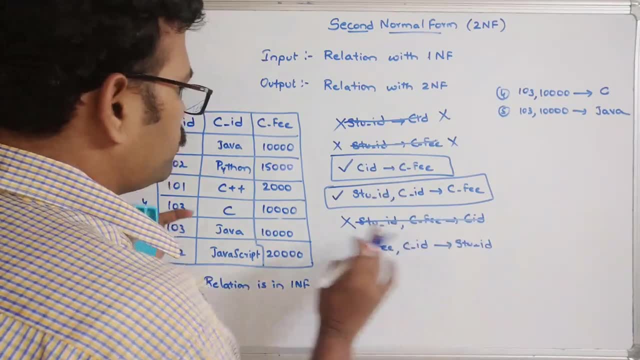 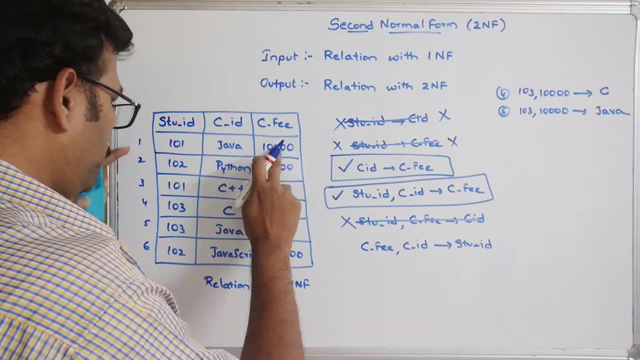 ID gives to student ID. Let us check course fee and course ID. So 10,000 in Java. Yes, Is there any repetition? Yes, 10,000 in Java. So first tuple and fifth tuple. So first tuple from first tuple. 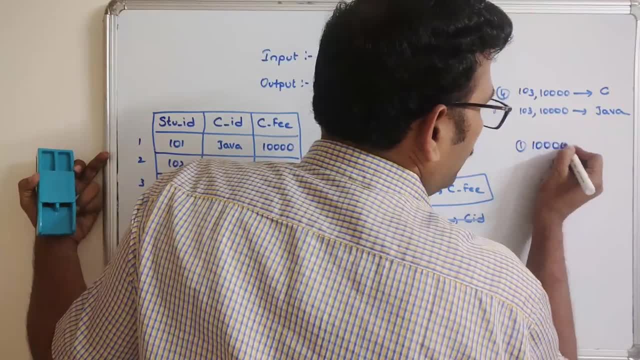 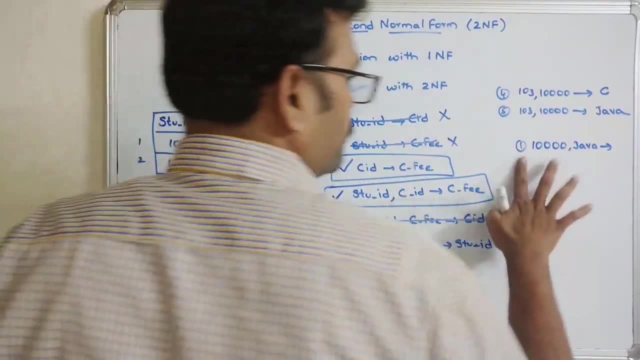 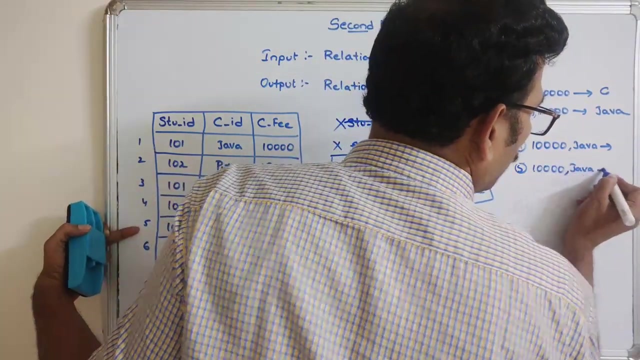 what is the thing? Course fee: 10,000 and Java. And next to fifth tuple: Yes, Fifth tuple, Fifth tuple. So fifth tuple is also gives the same thing: 10,000 and Java. So what about the Y values? Both. 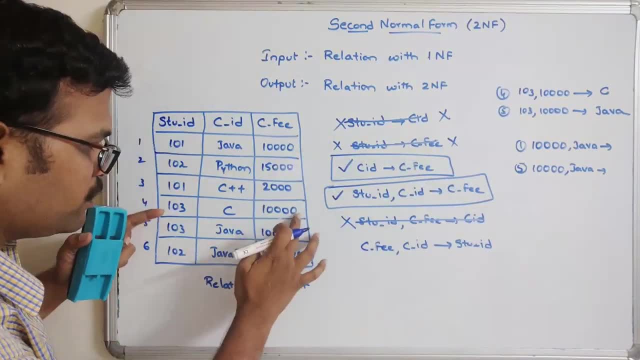 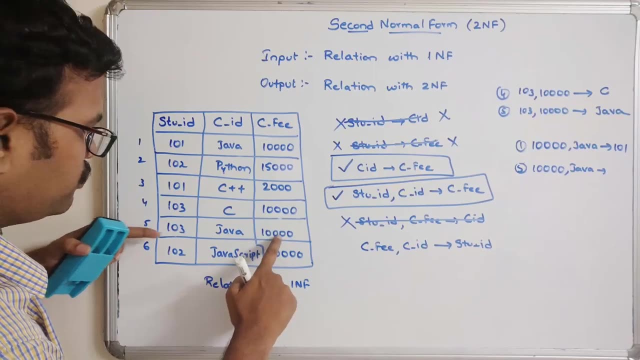 the both X values are same. What about the Y values? So Y values are so 10,000 and Java gives 101 student ID 101. And from the fifth tuple, again 10,000 and Java gives the student ID 103.. So for: 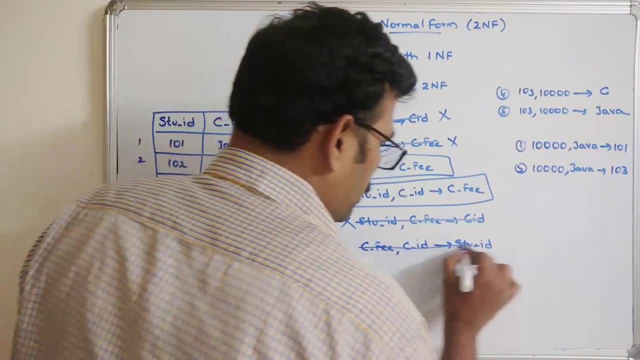 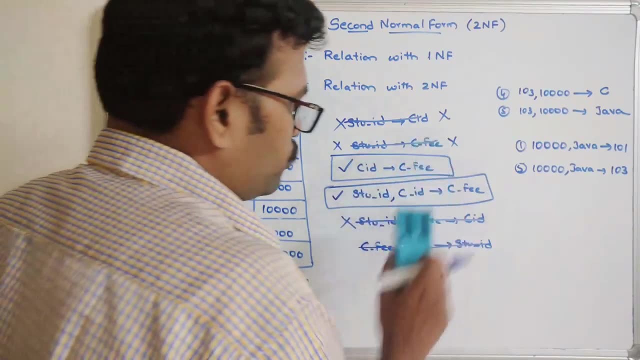 the same X value, there are different Y values, So this is also not correct. This is also not correct. I mean, this is also not a functionally dependent Now. so among these two we can consider the second one, because here we are having a set of attributes. 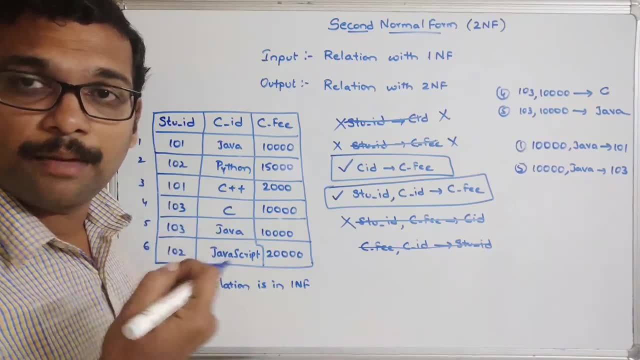 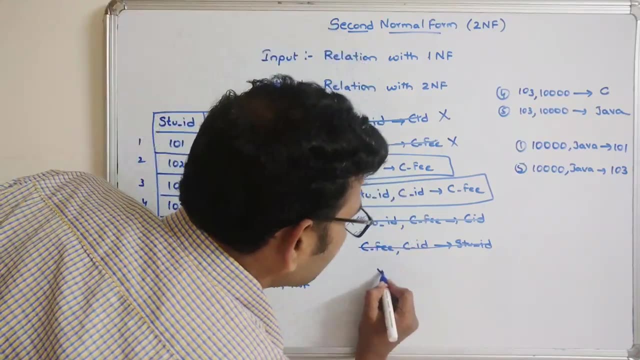 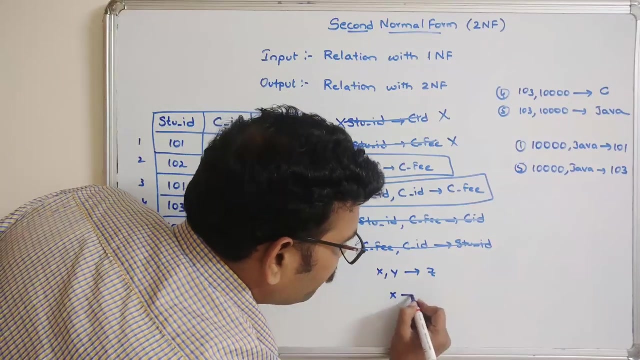 in the X value. That means a determinants. Okay, In the determinant- I mean in the determinant- we are having a multiple values. So this is like X comma Y tends to Z, See X comma Y tends to Z. So what we have done, So we have to check for X tends to Z and Y tends to Z, Whether these two are functionally. 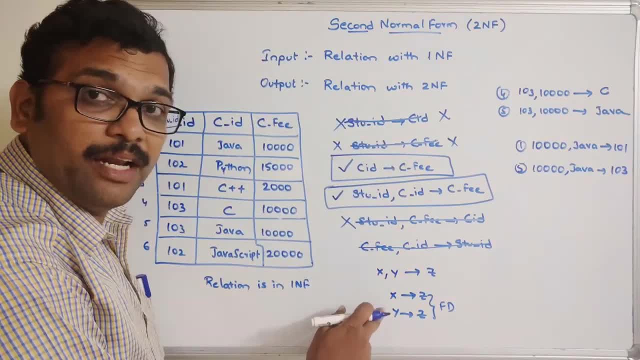 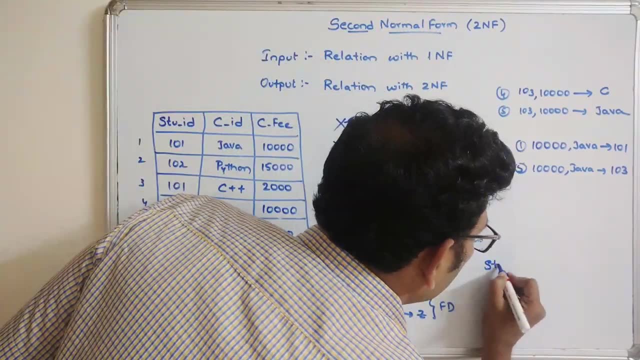 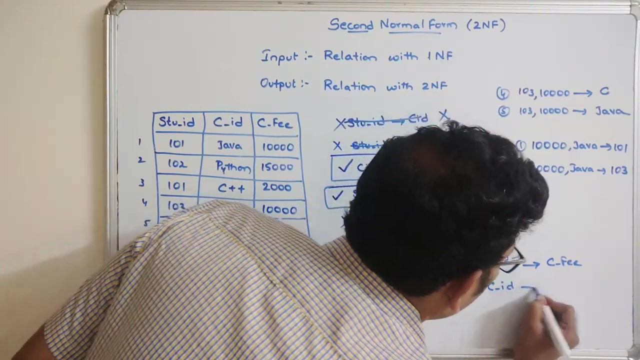 dependent or not. So if anyone of these things is a functionally dependent, we can say it is a partial functionally dependent. So now let us check. So from this one let us check: Student ID gives a course fee. similarly, course ID gives the course fee. So if any one of these functionally, this functionally, 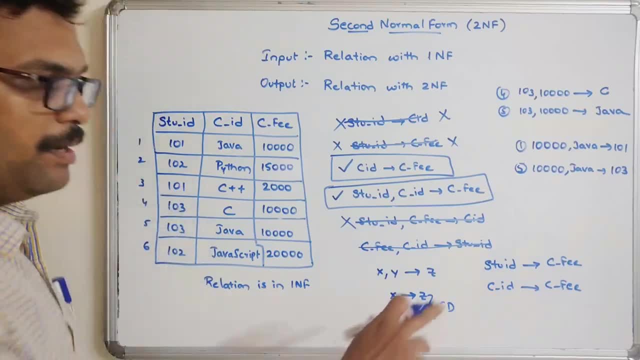 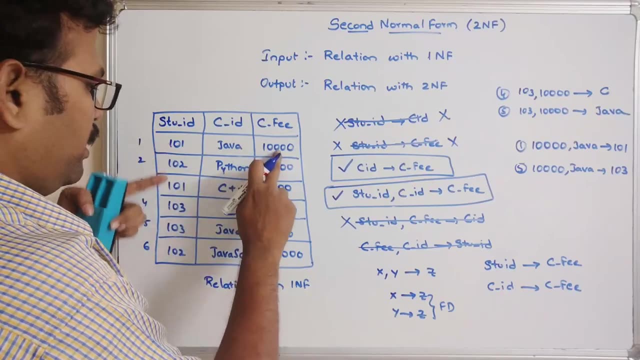 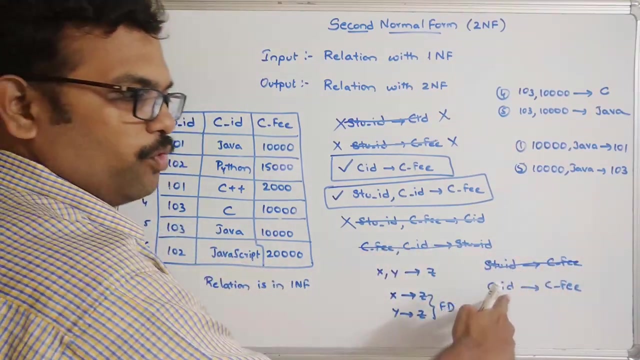 dependent. if this relation is a functionally dependent, then we can say it is a partial functional. student ID tends to course fee, student id and course fee. so 101, 10000 here, 101, 2000. so this is not a functionally dependent and coming to this, one course id tends to course fee. already it is a functionally dependent. 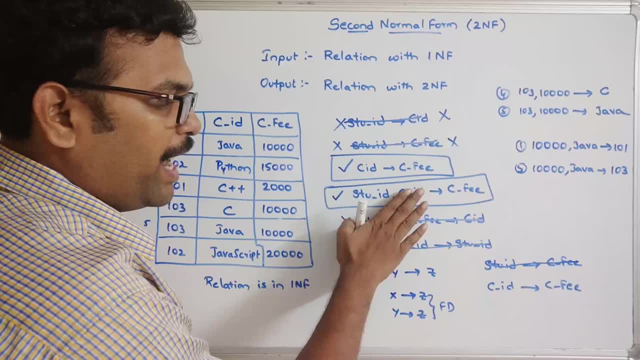 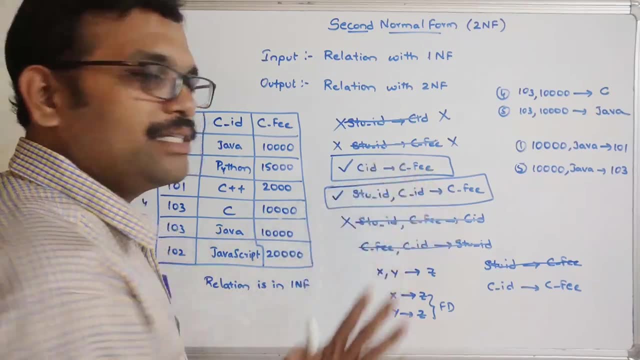 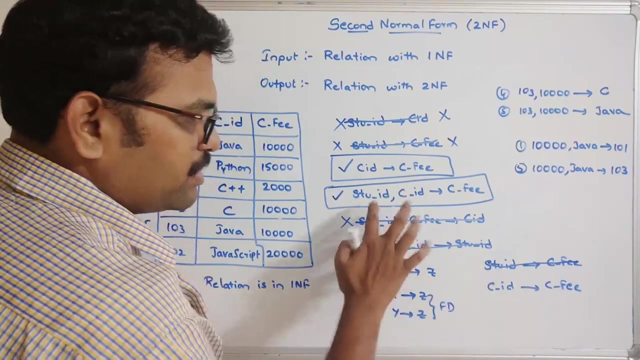 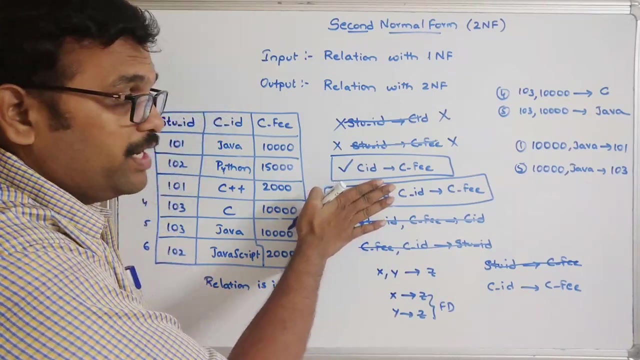 right. so here we are removing one attribute from the determinant. we are removing one attribute from the determinant, still it exists: the functionally dependent. so obviously it will be the partial functional dependent. so here we. in this case we are checking for both the cases. that means we are removing one attribute and we are checking for the functionally dependent. so 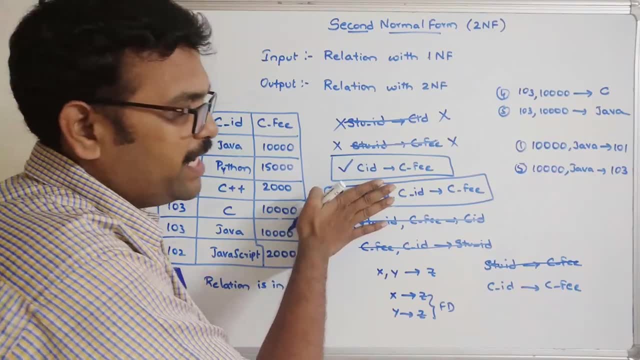 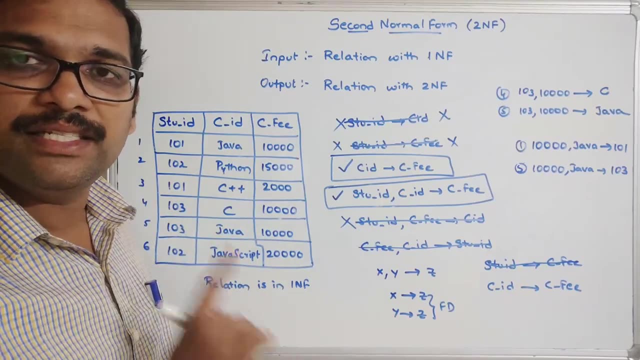 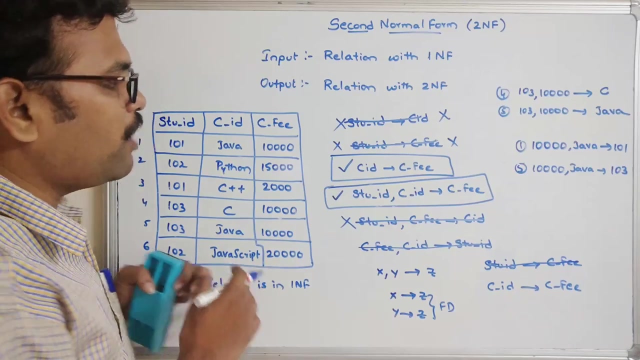 it satisfies the functionally dependence concept. right then we can say it is a partially functional dependent. so this relation is having partial functional dependency. so that means this is not in to nf. this is not in to nf, so how we can get this to nf? so we have to. 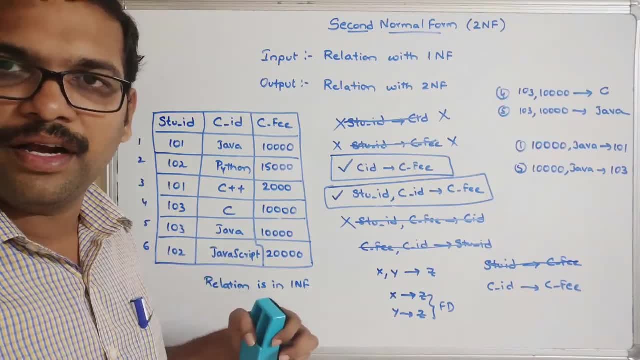 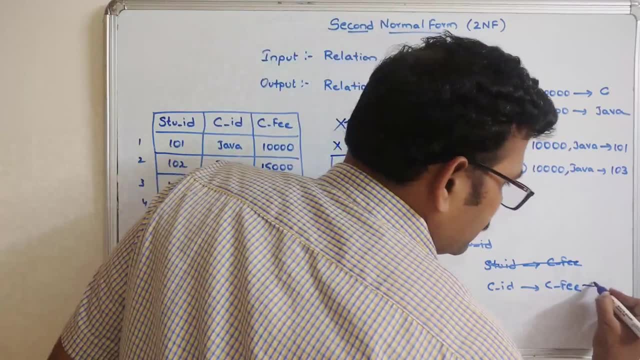 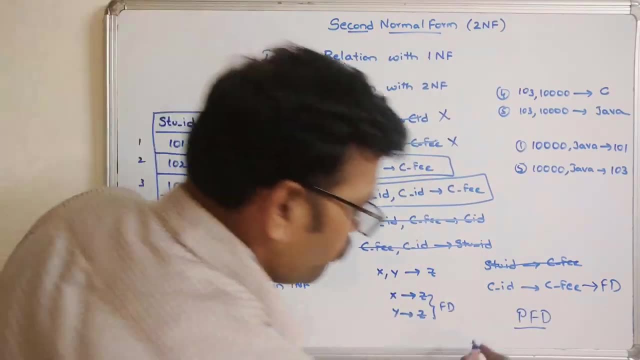 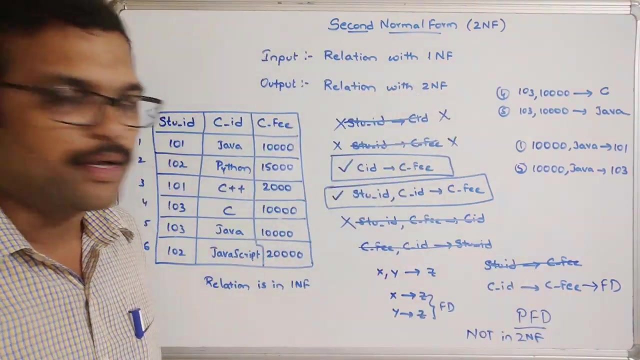 to two different relations. so this is a functionally dependent. so obviously we can say it is a partially functionally dependent, partially functionally dependent. so we can simply say not in to n f, not in to n f right. so now we have to divide or decompose the relation. 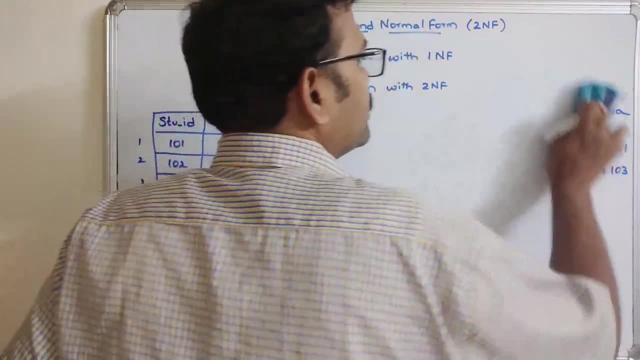 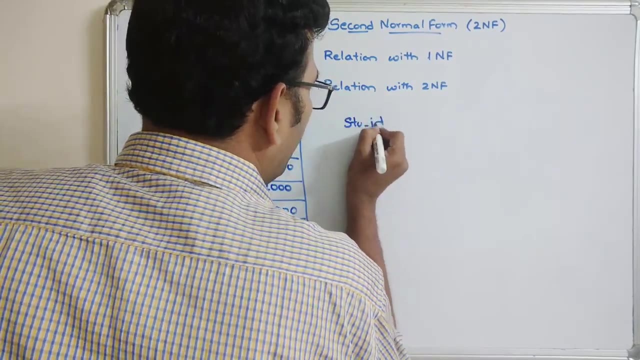 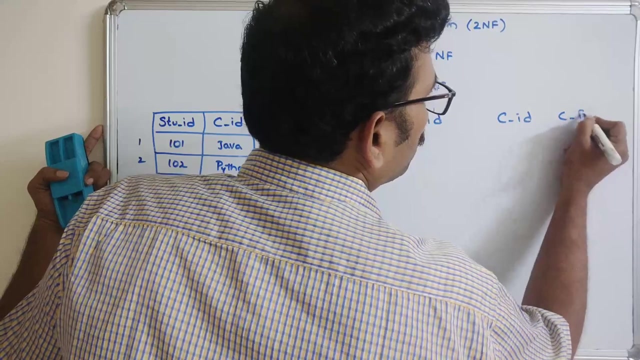 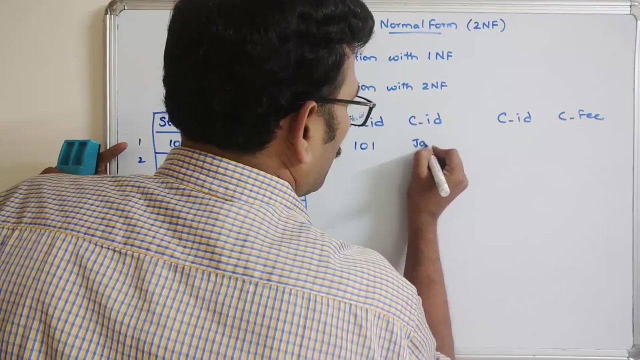 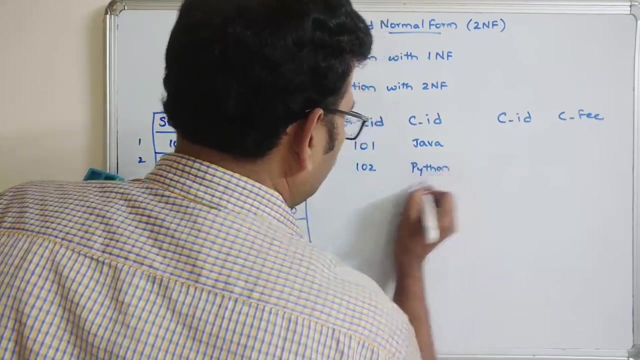 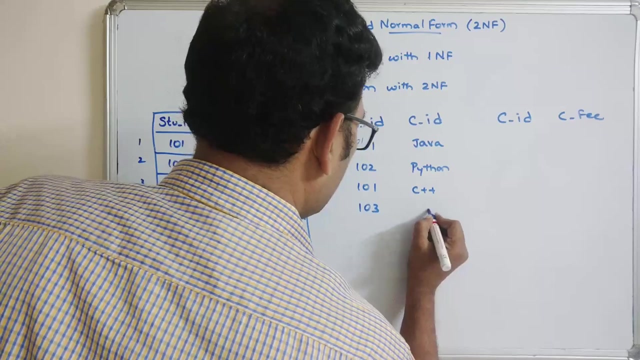 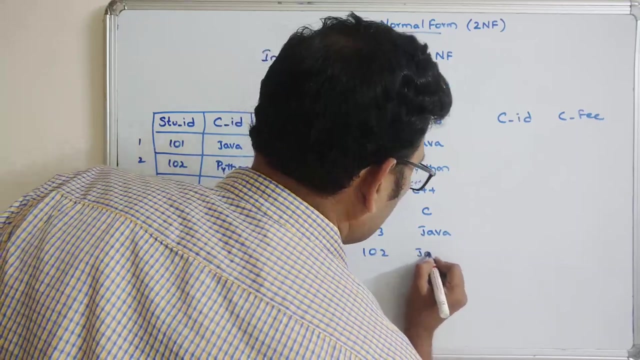 to two different relations, sub relations. so what are the sub relations? where we got that this one? so student ID and course ID is one table. course ID and course fee is another table. coming to the student ID, so 101 Java 102, Python, 101 see plus plus. 103 see 103 Java 102, javascript. so this is one. 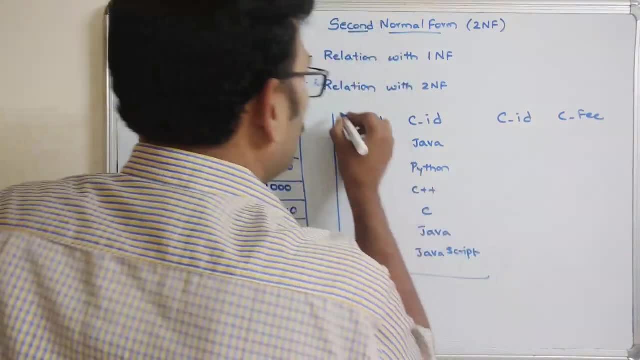 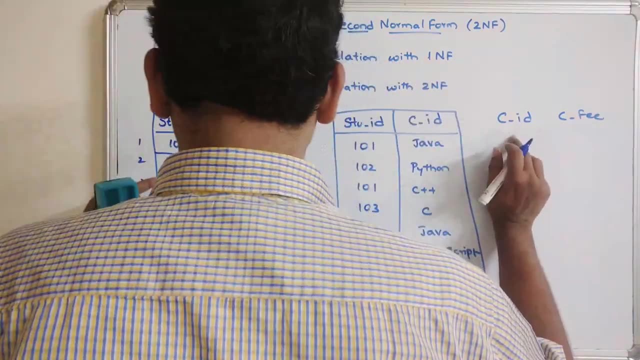 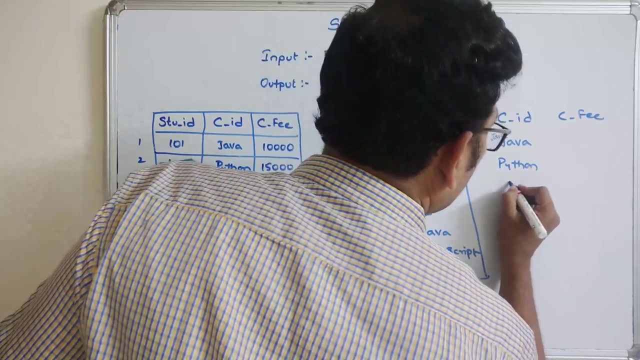 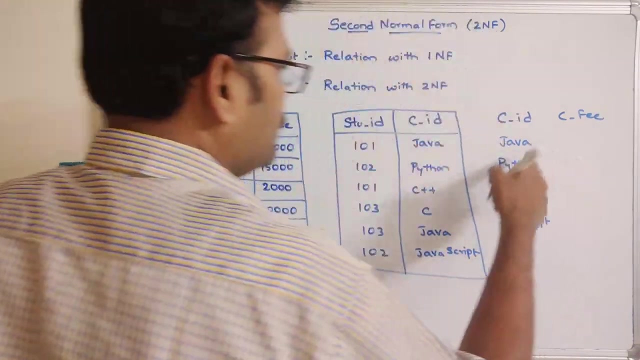 relation. there is a only one relation. okay, we are decomposing the complete relation into two sub relations. this is one relation and course ID. so I Java Python, C++, C, JavaScript, so here there will be no redundancy, you can observe. so we are having some six tuples, but here we are having only five tuples. 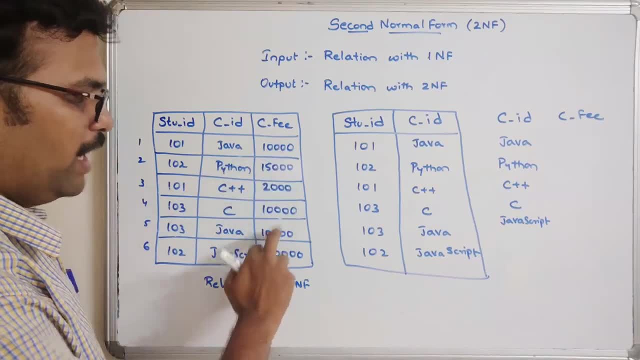 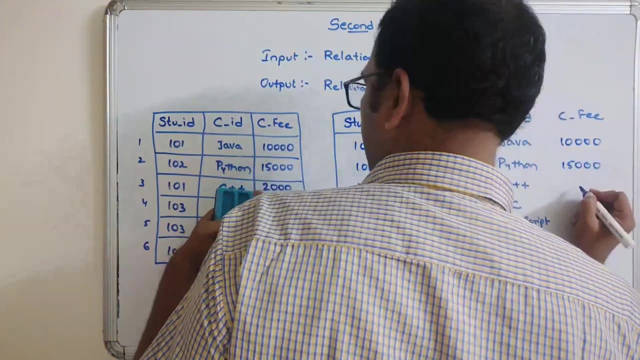 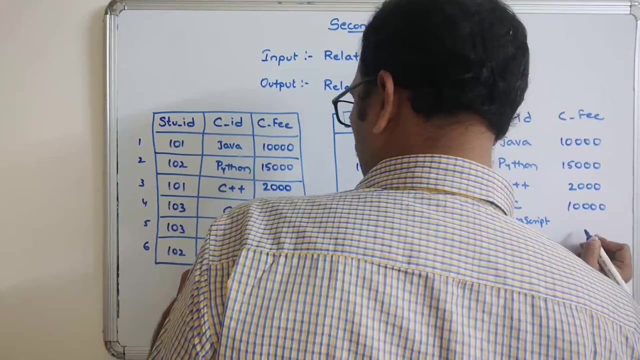 because Java is repeated, the same course, we value, same course. we value so, which is a 10,000, and for this one, Python, it is a 15,000 and C++ is a 2,000 and for the C it is again 10,000 and for JavaScript it is a 20,000. so you can observe here. 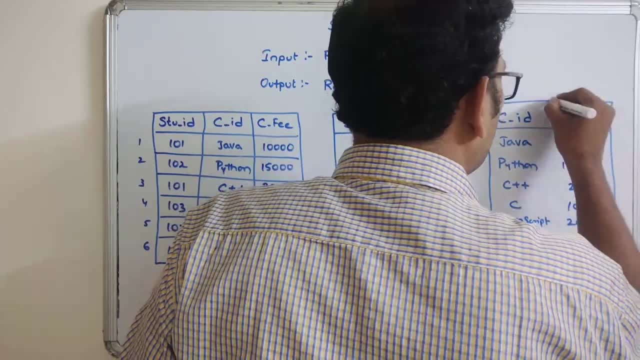 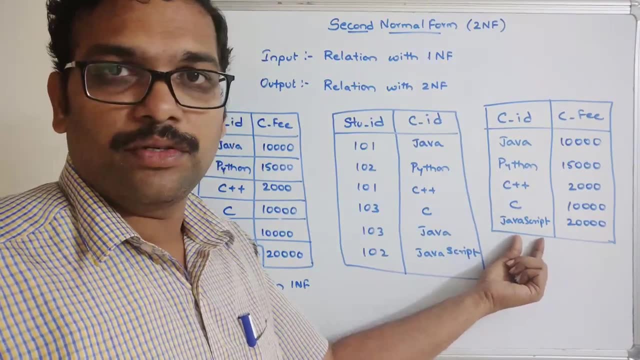 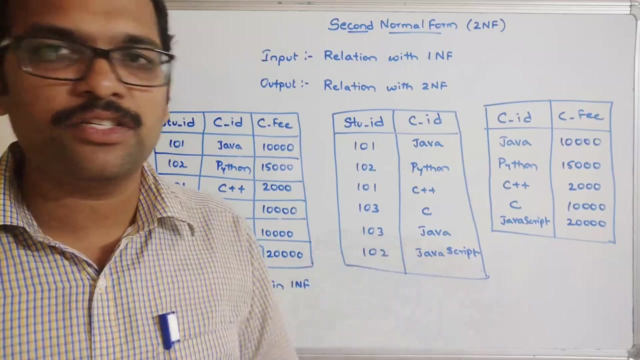 some sort of redundancy has been reduced, right. so here we are having some six columns, and here we are having some five columns. I mean five rows, rows, right. so like this we have to decompose the complete relation into a sub relation. so now you can say these two relations are in 2NF. 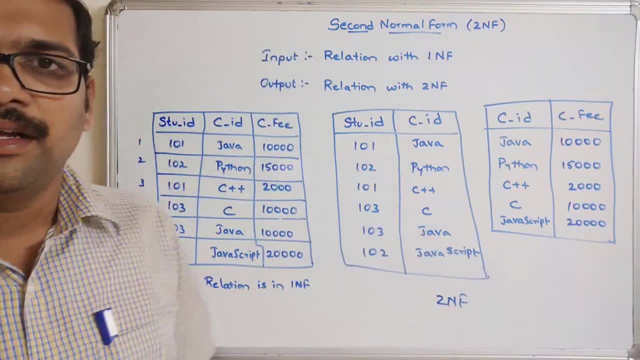 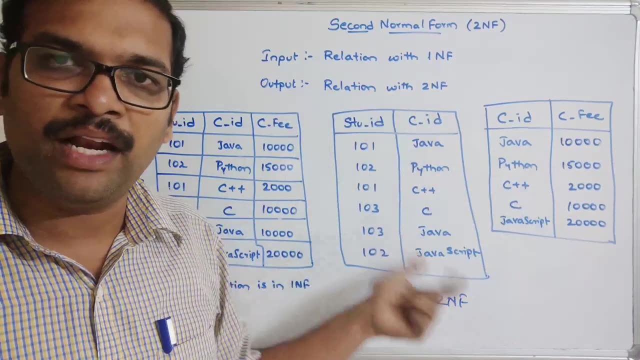 because there are no partial dependencies. so again you can check for 1NF and 2NF for this particular subrelations, if there are more number of attributes. and again you have to check for 1NF or 2NF. so whether it is 1NF then we have to check for 2NF, right? so again you have. 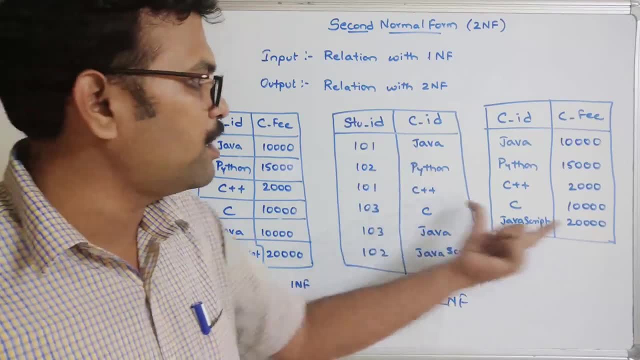 to check for partial dependencies, whether there are any partial dependencies in this particular sub relation or not. so if there are any partial Pf Smells. now there is a new reference for two nf, so I will suck a asts right, you should now check each one of these people because they testing. 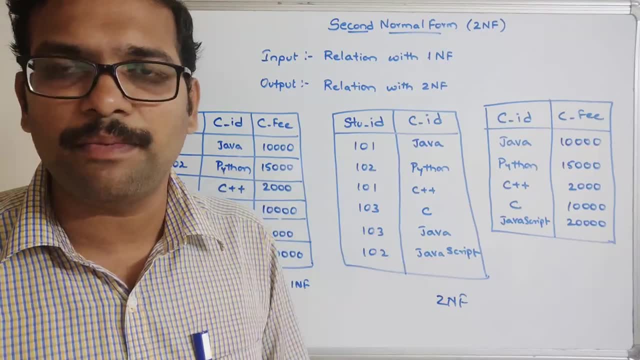 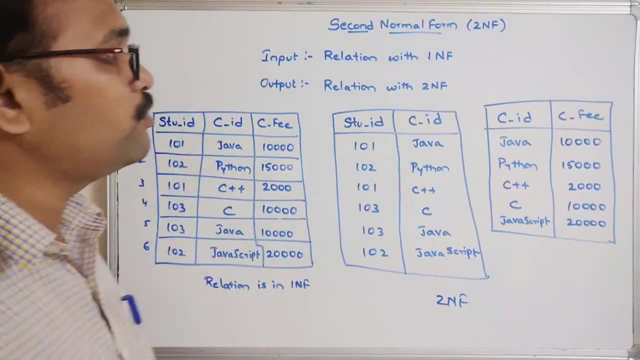 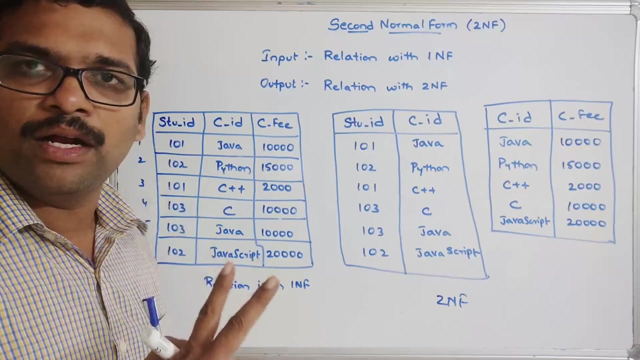 for any partial dependencies, as long as it does not incluides any singular subrelations, functional dependencies, automatically we have to remove those partial functional dependencies. that means by decomposing further, decomposing the relation into sub relations. so this is how we we have to satisfy the relation with 2nf- the first one. the relation should be in 1nf- the second one. 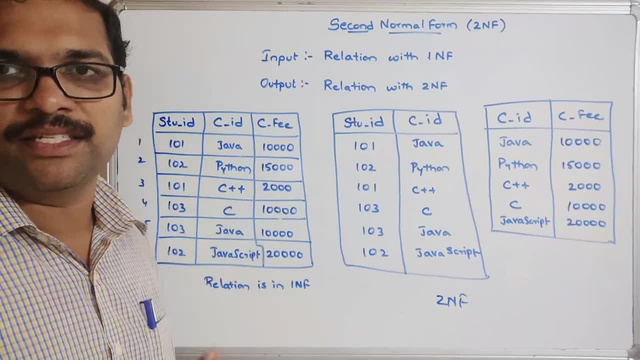 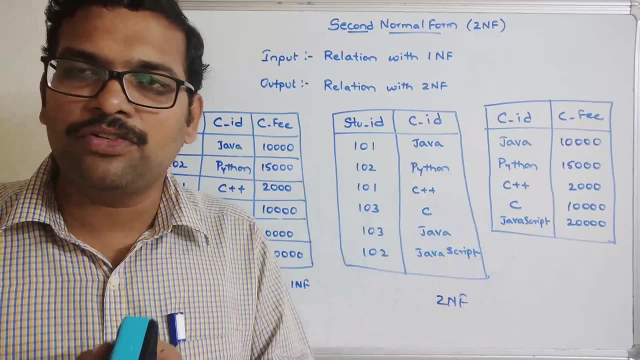 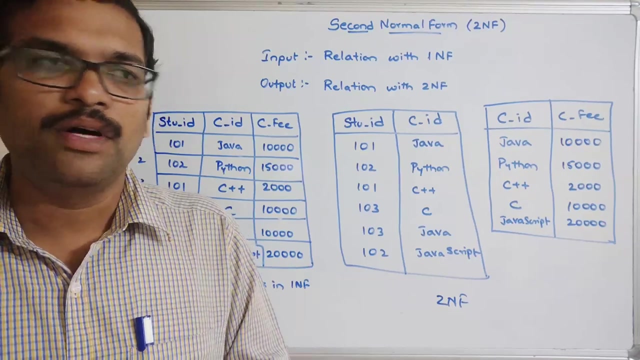 the relation should not have any partial functional dependencies. so once again- and i am saying that the just view the links of partial, i mean functional dependency concepts, so i will give the complete playlist in the description section. go through that, so listen to the functional dependency concept. what is the functional dependency and what is the full part? full? 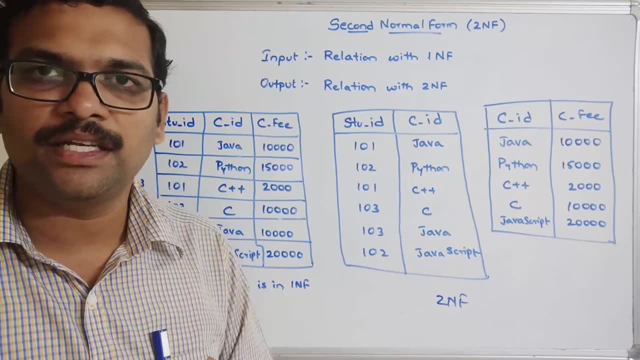 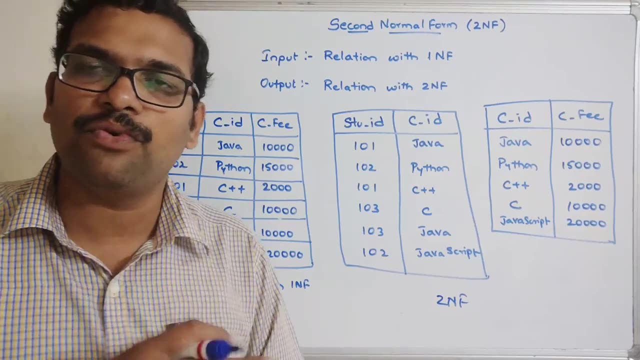 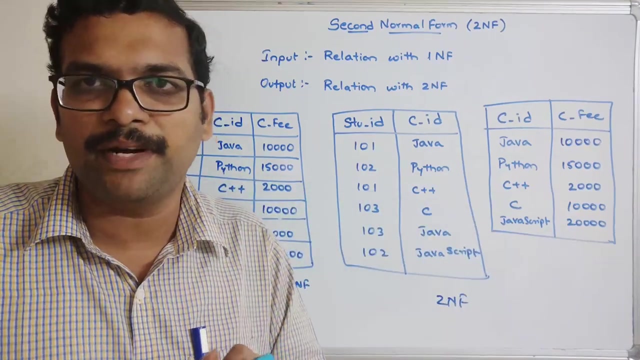 functional dependency, partial functional dependency, types of functional dependency, and then it would be very easy for you to understand this particular normalizations concept. so either it is 1nf, 2nf, 3nf, 4nf, etc, etc. so first visit the functional dependency make, just understand the concept of functional dependency. 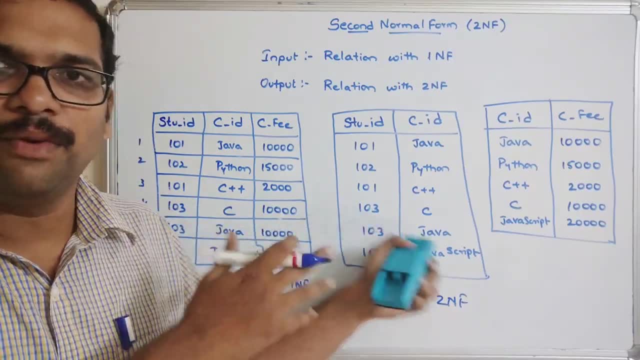 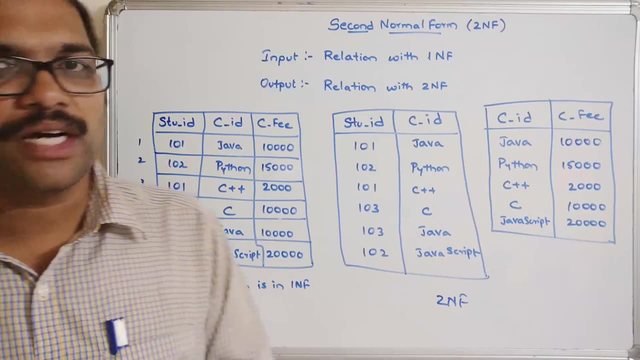 so it will be very easy for you, right? so the link will be given in the description, so go through that one before watching this video, right? so hope you understood this one, and if you are having any doubts regarding this second normal form, so feel free to post your doubts in the comment section. 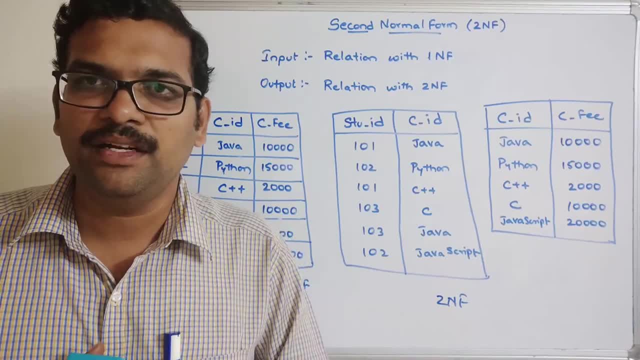 definitely. i will try to clarify all your doubts. if you really enjoyed my session, like my session, share my session with your friends and don't forget to subscribe to our channel. thanks for watching. thank you very much.